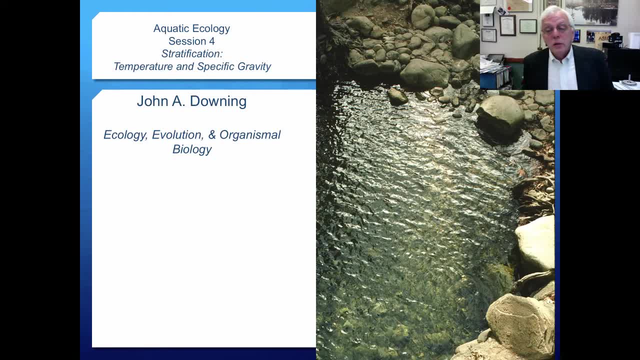 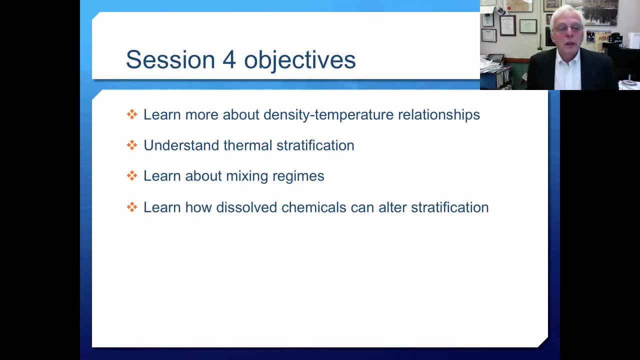 like to elaborate on that and tell you a little bit about why it's so important and what that means for aquatic ecosystems. So my objectives for today, this particular session, would be to have you learn more about the density- temperature relationship in water and understand thermal stratification in, especially in lakes or virtually any other kind of aquatic ecosystem, and then learn 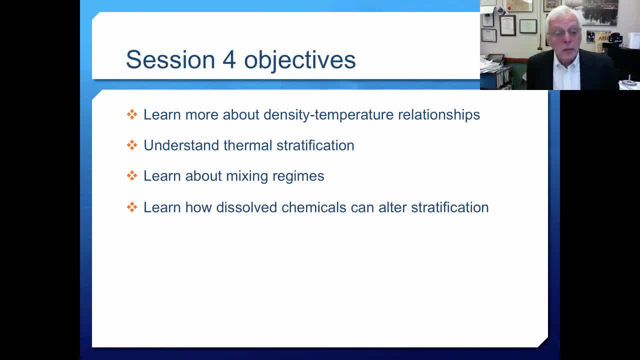 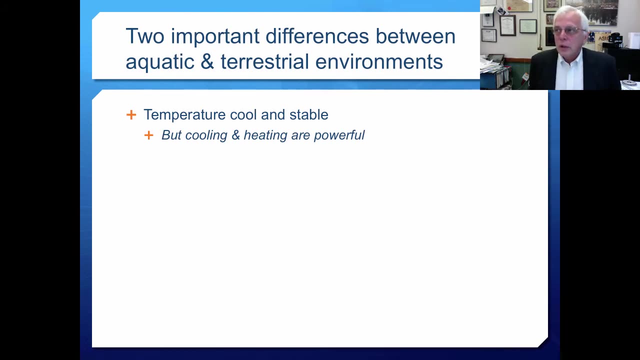 about mixing regimes- how how systems mix and when they mix- and then learn how dissolved chemicals can alter stratification. Those are my objectives and I hope that they work out for you. There are two important differences between aquatic and terrestrial environments, and these are we're. 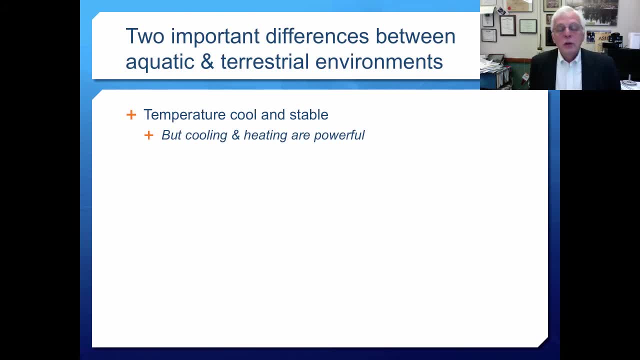 going to talk quite a bit about these over the next two sessions. First, an aquatic environment or ecosystem. in an aquatic ecosystem the temperature is pretty cool and stable, that is, to be moderated, and this is due to the specific heat and also the heat of vaporization of water. and 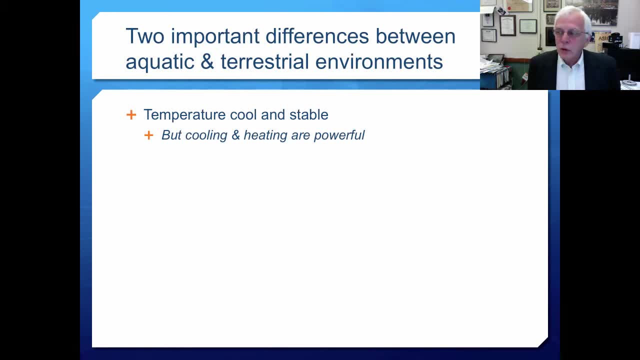 cooling and heating, however, are very powerful, and you know this if you've ever stayed too long swimming in a cool, a cool lake. And the other important difference between aquatic and terrestrial environments is that the light environment is modulated by water, modulated, moderated by water. 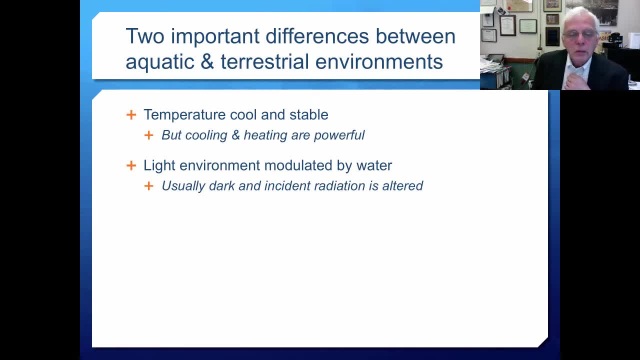 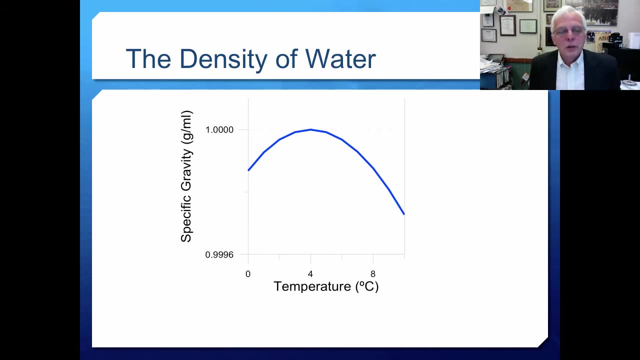 It's usually dark, relatively dark relative to terrestrial environments, and incident radiation can be altered, and these would be the topics over the next couple of sessions. Now you will recall that we talked about one very special aspect of water, that being its specific gravity or density, here showed in shown in grams per. 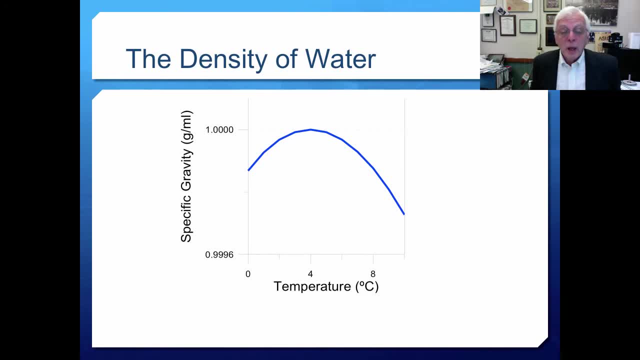 milliliter or grams per cubic centimeter roughly, and on the x-axis, you know, there's temperature and we're only over a range of temperature from zero to ten degrees, Ten degrees being rather cool water to go into. so that would be something for those of you do Fahrenheit somewhere in the 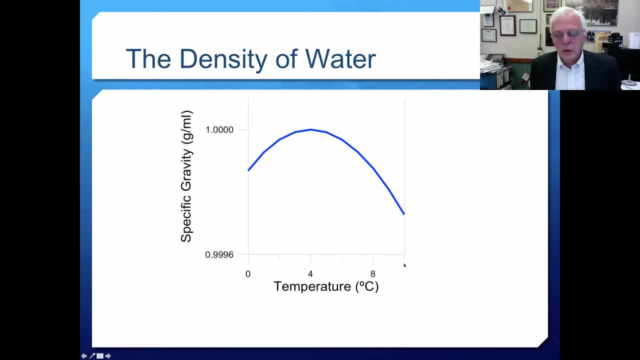 range of fifty five degrees at the upper, or maybe fifty degrees at the upper end of this, of this graph, and zero is of course the point of freezing of water, and here's a specific gravity, and you'll note that it hits a maximum at about four degrees Celsius and that we discussed already in the. 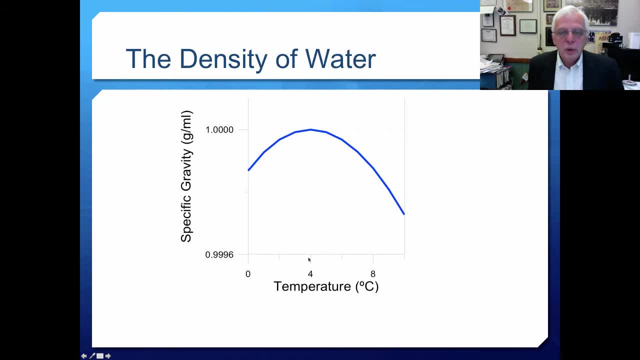 miracles session, So you should be pretty familiar with this idea. Now, the important thing is that the important part of this is, of course, that water that's four degrees Celsius is going to be the heaviest per unit volume of any water in the system, and this has very important implications. 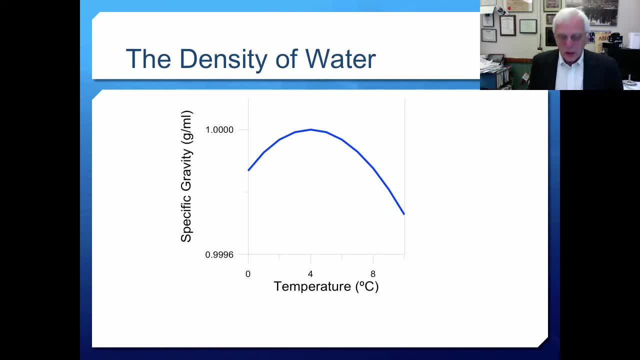 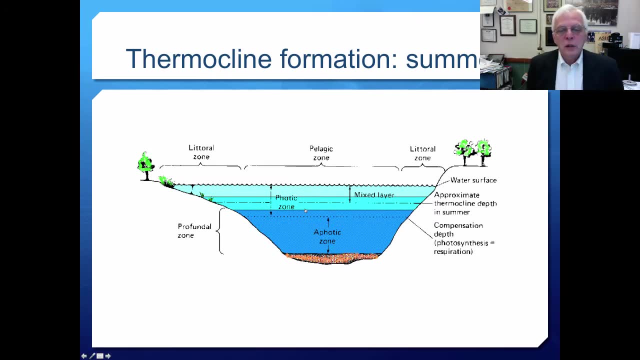 of course, for for stratification of lakes and ponds, particularly So in the summertime. there is a thermocline that's formed, and thermocline is an area of very rapid temperature change and you can feel this yourself if you go swimming and dive down, kind of. 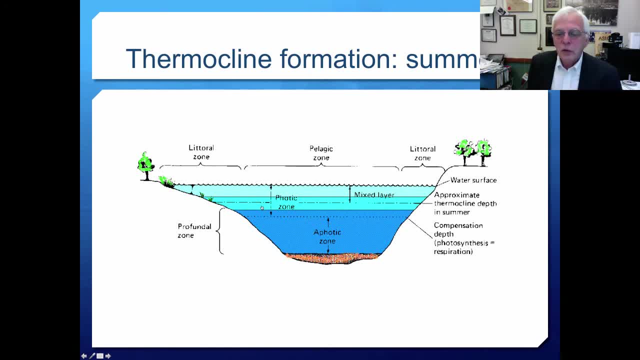 deep in a lake and somewhere around 10 meters or about 30 feet in a fairly large lake, you should find an area in the summertime where temperature gets quite cool quite rapidly. Now what this means is the. the ecosystem is divided into basically three layers or three zones. One is the epilimnion. 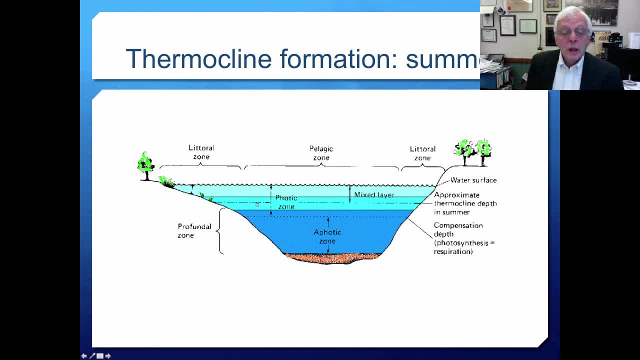 up here this upper water at the top of the system, The middle system is. the middle part of the system is where the temperature is and the upper part of the system is where the temperature is. So if you look at the bottom, you'll see that the temperature is changing rather rapidly. that's called the 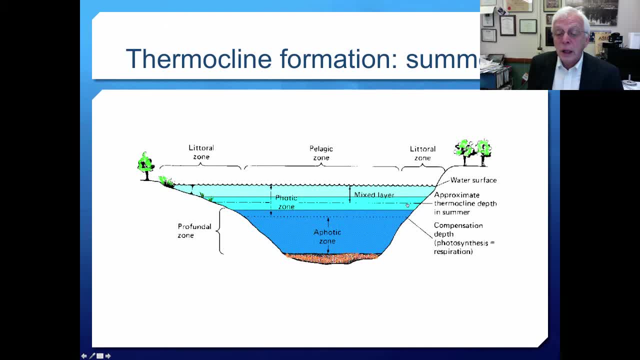 metalimnion, and in the middle of the metalimnion you find the thermocline, and down in the bottom you'll find the hypolimnion, or the deeper water. hypo, meaning under the lake, hypolimnion, be under the lake. Now, also on this figure, you see things called photic zone, a photic zone and so on, and 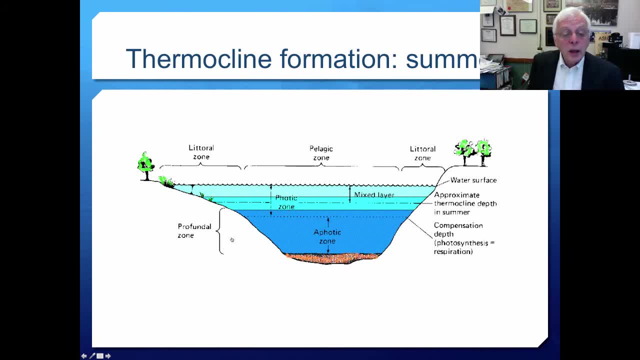 we'll get to those a little bit later. but anywhere down in the hypolimnion in a, a lake system would be called the profundal zone. anywhere up at the upper part of the metalimnion and the entire epilimnion is what we call the mixed layer and that water is mixing. 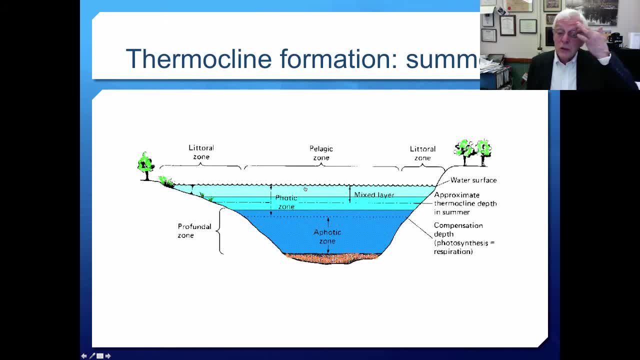 fairly continuously throughout this period of the summer. Now this is what it looks like in the summer and naturally down here at the bottom, the temperature is going to be the water that has the highest specific gravity. Water with the highest specific gravity is always somewhere around four degrees celsius and in effect it ranges from about four to six in deep lakes. that. 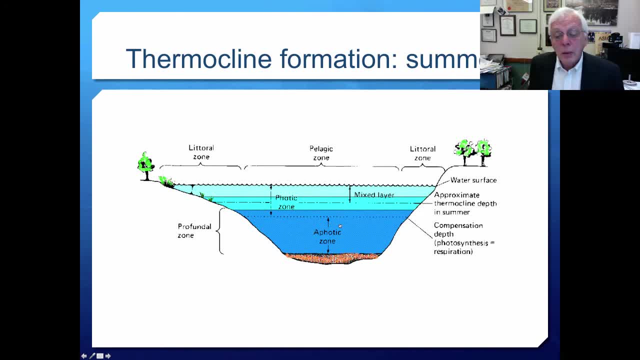 I work on in the temperate zone, So the hypolimnion is is always around four degrees celsius in the summer, unless there are period. there's periodic mixing and warmer water is mixed down into the hypolimnion. The upper mixed layer will be somewhere approaching ambient, but as you know from 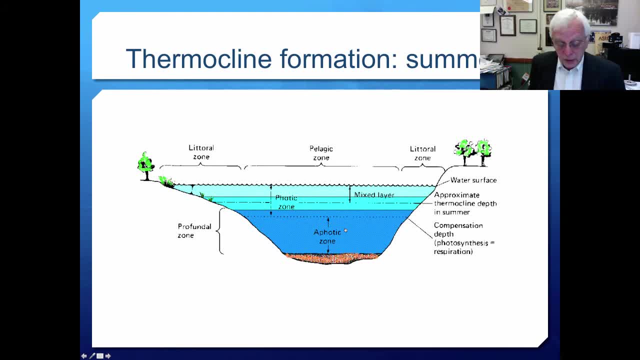 the heat of vaporization of water. it's probably not the other way around And it's going to be some a little helplessness from time going to be up in the high numbers that you see for air temperature. so that's what the thermocline looks like in the summer, and now here's what it looks like. 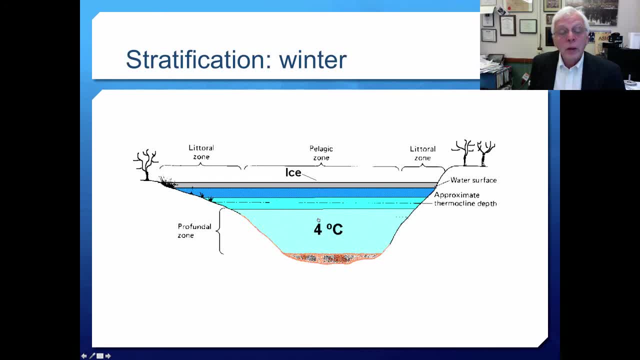 in the winter. recall, then, that water with a with a specific gravity, with a temperature of about 4 degrees Celsius, has the highest specific gravity of any water that you can have. therefore, in the winter time, the water is going to be rather warmer at the bottom than at the top. you can see in it. this is a 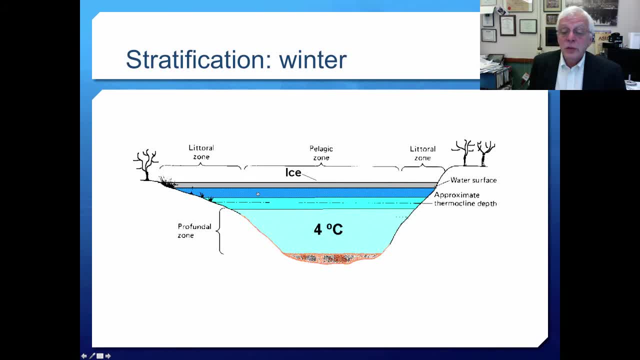 temperate zone lake. so here we have ice, ice formation. at the surface we have an epilimnion. it's definitely stratified. it may not be terribly strongly stratified in the winter time, but the stratification is held by ice. here's the metal imni and again in the middle the thermocline. here where we have the most. 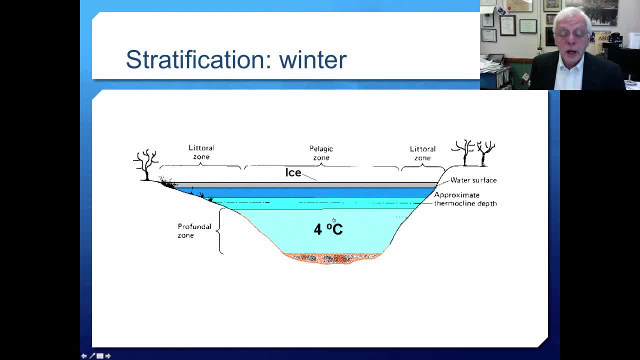 rapid rate of temperature change and then, down at the bottom is a hypolymni, and the hypolymni is 4 degrees, around 4 degrees Celsius. now, what that means is actually, if you've been thinking about what you saw in the previous graph and what you see, 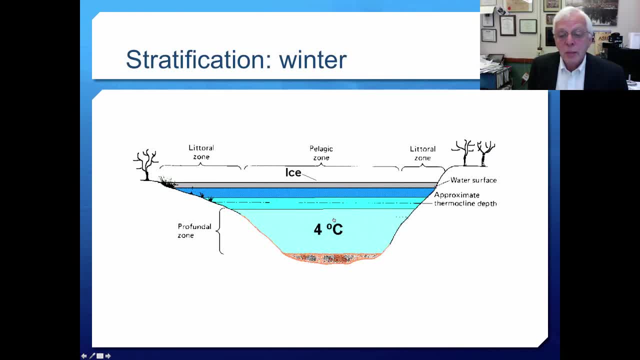 here. water at the bottom is almost always the same temperature in a deep zone, deep lake, in the temperate zone. this is obviously not true for for tropical lakes or subtropical lakes, but it certainly approaches truth for any way for stratification in the temperate zone and even in some of the 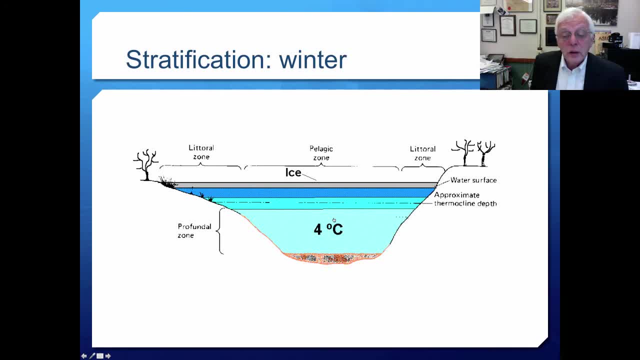 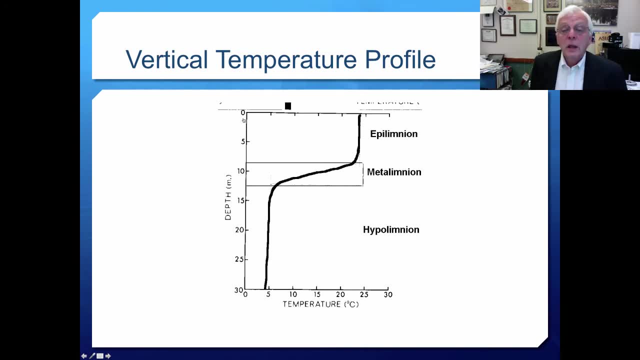 very well in the very high latitudes, until the lakes are permanently frozen. now this is a way that limnologists like to look at temperature data, and here, on the x-axis, you see temperature, here on the y-axis, you see inverted depth. so basically you can think about this as the top of the graph is, at the top of 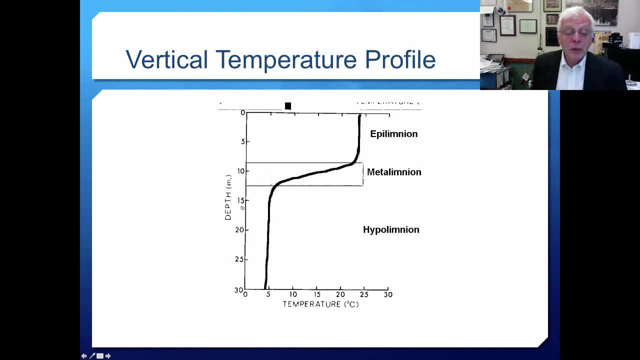 the water 0, 0 meters of depth. bottom of the water is at the bottom of the graph and then you see what the temperature looks like when you graph it. so to high temperature up in the 20s, clearly a summer, like summer or late spring or early fall kind of temperature. 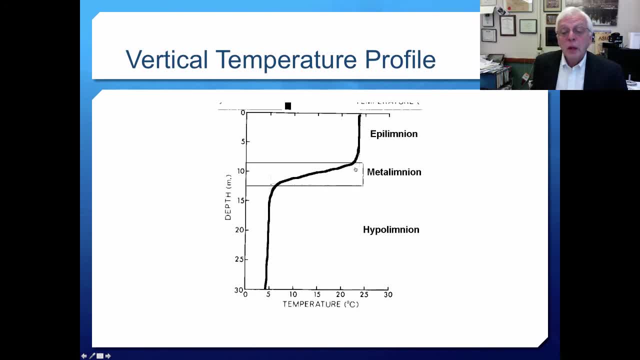 curve. but we here, we have the epilimnion, then we move into the meta limnion, which is the area of rapid temperature change, and then down into the hypolymni and which is the part of the lake that during stable, stable periods, does not. 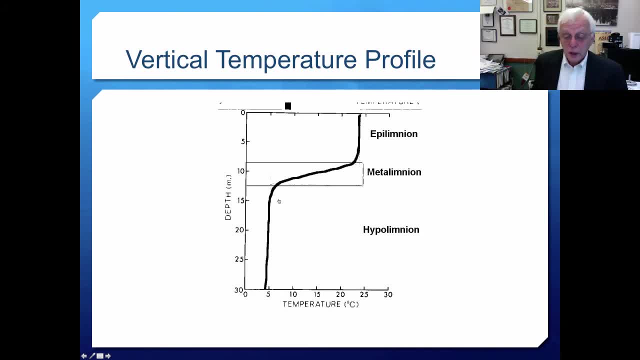 mix back into the rest of the water column. this is a typical way to see a water temperature profile. in a way, that's quite useful because you can see where the mix zone is easily the epilimnion and the upper bit of the metal imian, then the area of rapid temperature change somewhere in the 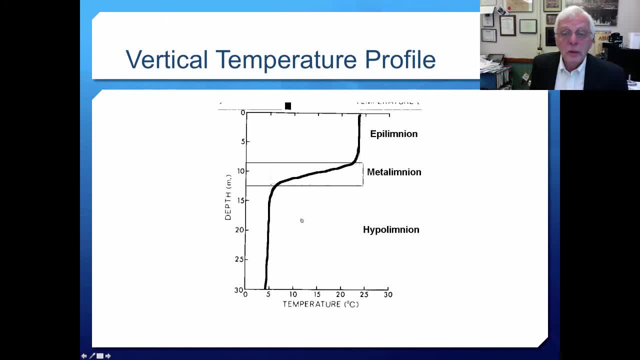 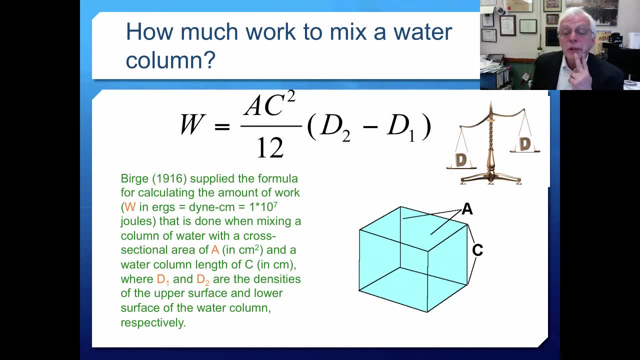 middle here would be the thermocline. at the bottom would be the hypolymnia. now you might ask yourself how much work it takes to mix a water column and that can be easily calculated with this kind of equation. this was actually put together by a very 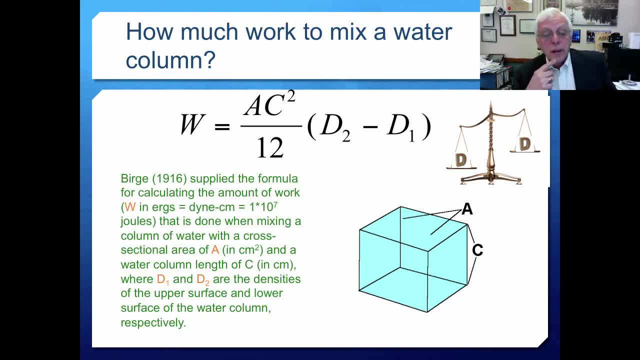 famous limnologist at the University of Wisconsin in the early nineteen hundreds, and W is the amount of work that is done when mixing a column of water with a cross-section of a in this cross-sectional area of a, which is measured in square centimeters, and a water column length of C, which is the. 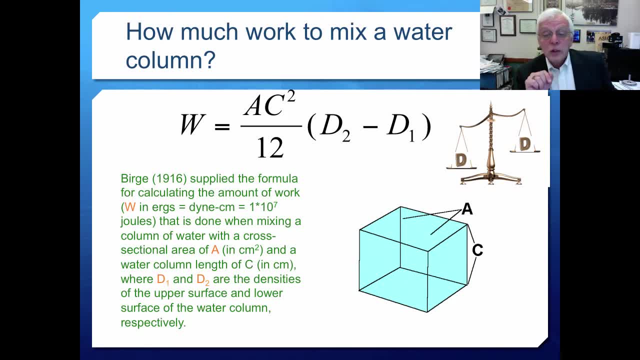 distance. you can see it in the cube over to the right so that you can visualize this now. d1 and d2 are the densities or specific gravities of the upper surface and lower surface of the water column respectively. so 1d is slightly more dense than the other. of course, my balance in the upper right. 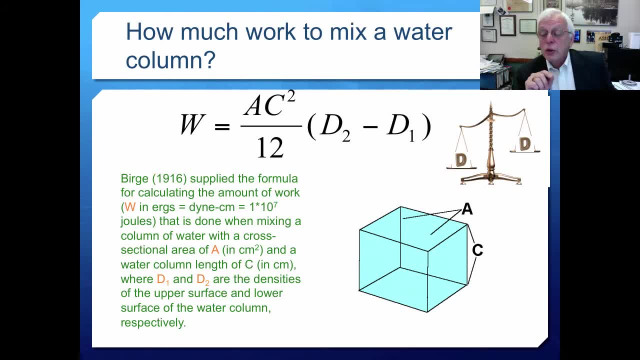 shows that one's heavier. in fact that is true if the given, if the volume is the same. so the densities are simply the categories, only specific gravities of the upper and lower part of that water column. now we can fiddler around with this equation pretty easily. now let's us see. 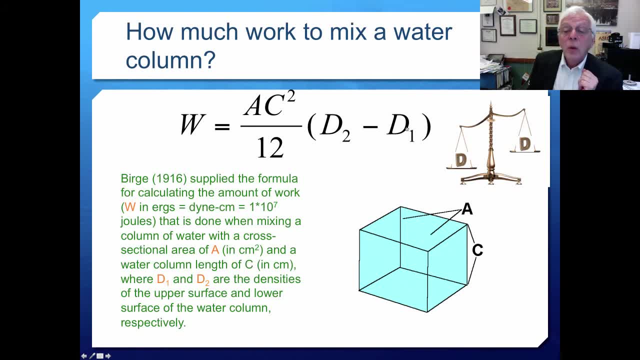 that we we work with the density's. now, when the densities are substantially different, of course you can see the difference will be much higher and this will be bigger multiplier of the rest of the equation, which leads to an increase in on equal 47 percent in terms of clean water. 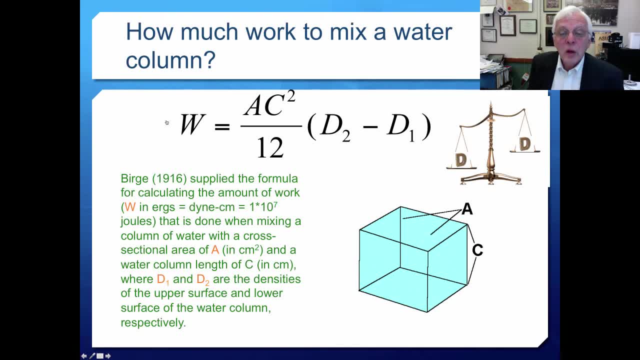 amount of work necessary to mix the water column. very straightforward, isn't it? so the greater the curve of change in specific gravity with change in depth, then the higher the stability. that is to say, it takes more work to mix the water column. um, now, if we're thinking of an area of a small cube of water and say a 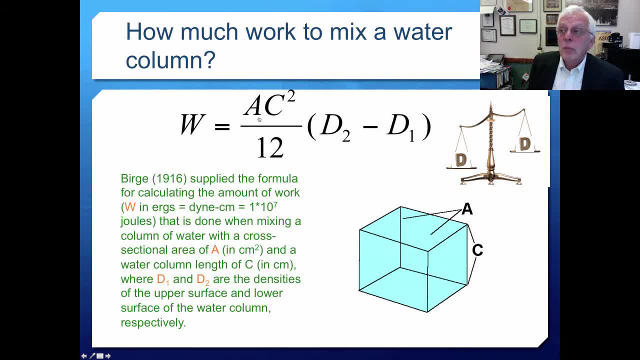 few centimeters, or an entire lake, which will be many, many square meters the lake. the bigger number, the bigger the measurement of a, then the greater the amount of work. so a bigger ecosystem takes more work, more energy to mix it, the water column, then then a smaller one or a smaller piece of water, and likewise. 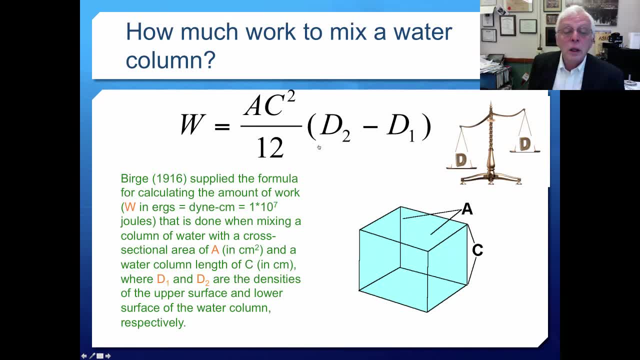 the depth over which you're considering mixing the water column. the work increases as the square of that depth. so it takes a substantial amount of more work to mix a, let's say a, a deep thermocline and a deep metal imnion and hypo limnion. then it would take to mix a. 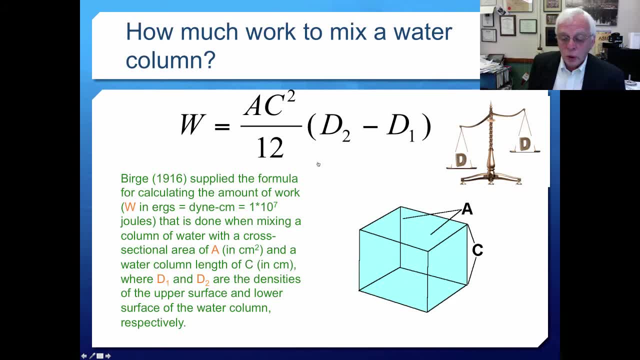 really shallow one. so all of these things go to the amount of work we have to put in in order to mix that system. now, sort of the you inverse way of thinking about that is that the amount of work it takes, uh, is also proportional to the stability. 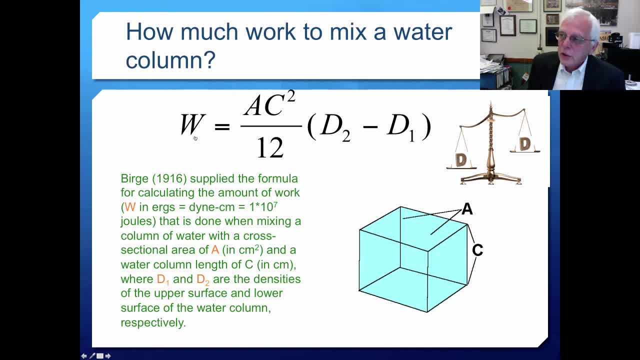 of that, the relative stability of that water column. some cases we may have a very stable water column, others it may not be terribly stable, and that all depends on the amount of work it takes, which depends, of course, on the rate of the rate of change in um a specific gravity of water, with with depth, as well as the size of the. 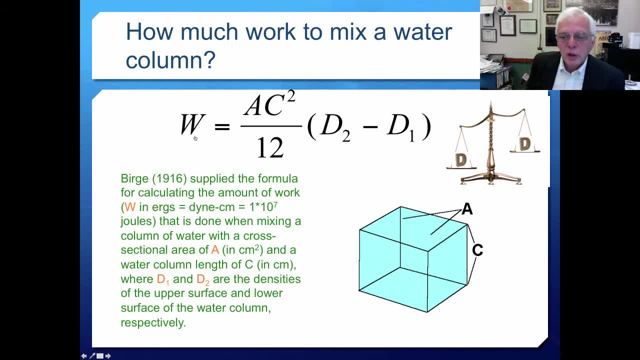 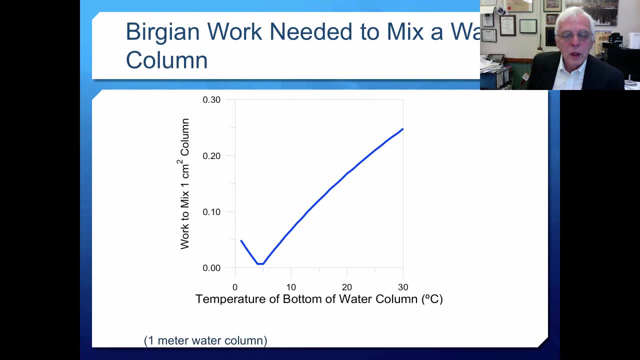 the system and the depth of the ecosystem. very straightforward equation. you should probably work with this a little bit just to get familiar with it and think about it, because it has a great it's. it's really important for to understand when an aquatic system might mix. now, before when we looked at the 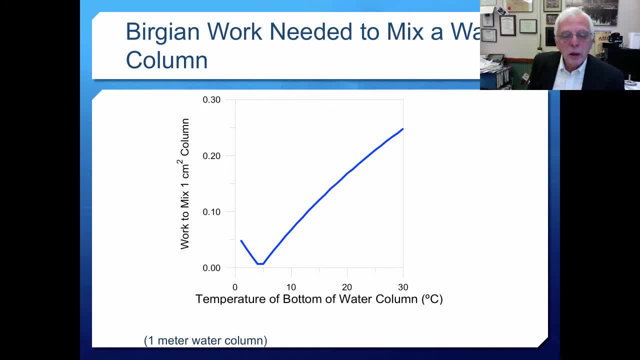 same curve. we were looking at the, not the amount, not the temp, not the amount of work it took, but the actual differences in stability. and this is what. but right here, what you're seeing is the work needed to mix once one square centimeter water column that is one meter deep, just as an example. and 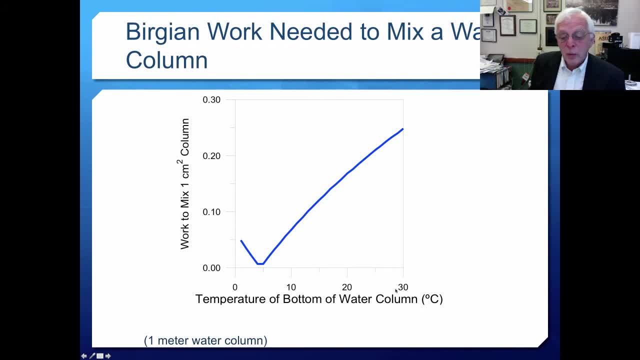 this is the temperature of the bottom of the water column, where we have a rate of change of one degree Celsius per per meter. what you can see from this, I hope, is that you can have extremely high rates of stability or a large amount of work needed to mix a water column when the temperatures are 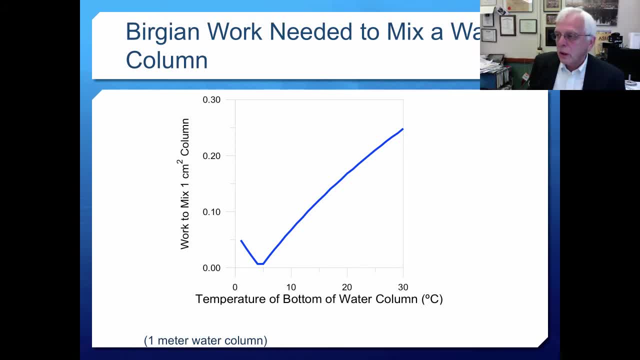 warm and this has to do with that previous graph that we saw the sort of accelerating change in specific gravity with with temperature. that causes um. that causes a great deal of stability to be possible in very warm systems. So you can often find microstratification even in the temperate zone. Sometimes you'll have 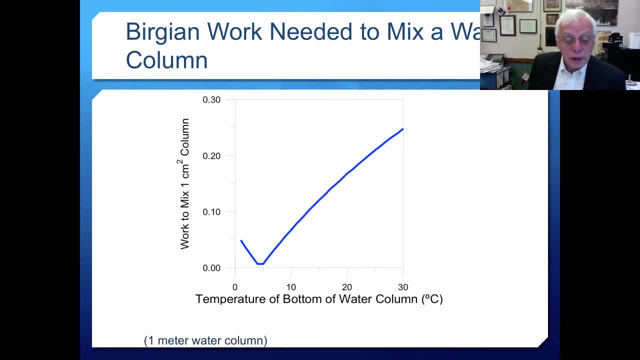 many small thermoclines, and that's because when water is quite warm then the differences in its specific gravity for a degree of temperature change is quite large. So this is the amount of work and this allows a great deal of stability, even in warm waters with small rates of change. 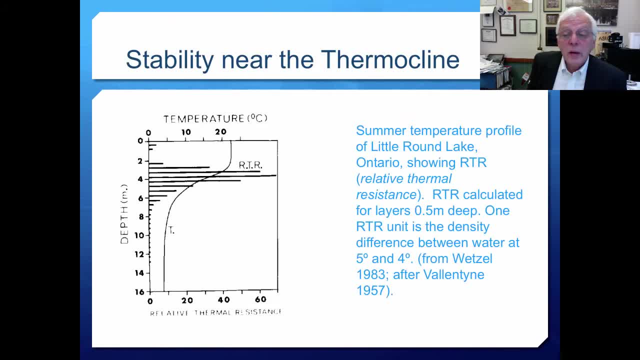 of temperature. Here we have the relative thermal resistance to mixing as a sort of a bar graph superimposed in on the same kind of temperature graph we were seeing before, And on the x-axis again you have both temperature but also relative thermal resistance to mixing, the RTR. 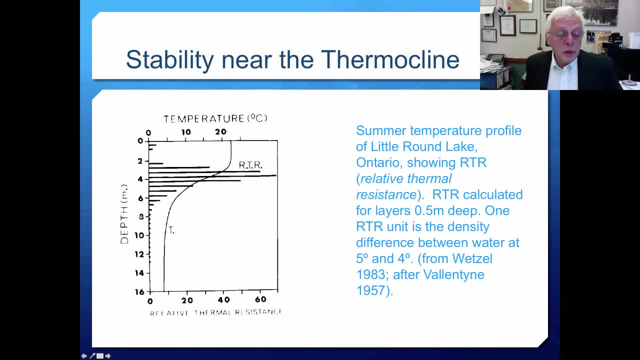 measure. And then this is, of course, depth 0 to 16 meters on the y-axis, arranged in the way limnologists like to arrange them. Here you see a little bit of microstratification in the upper waters, but where you really see relative thermal resistance to mixing is right at the thermocline. 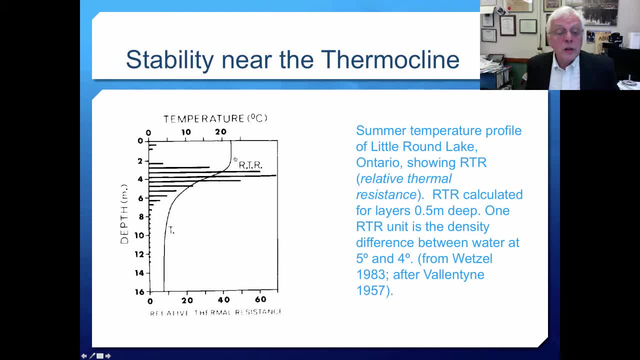 So this is all calculated for layers that will be a half of a meter deep, or about a foot and a half- anny, yeah, correct, half- in imperial units. one rtr unit is the density difference between water at five and four degrees, and this is um. this shows you a one way of determining where the actual thermocline might be. 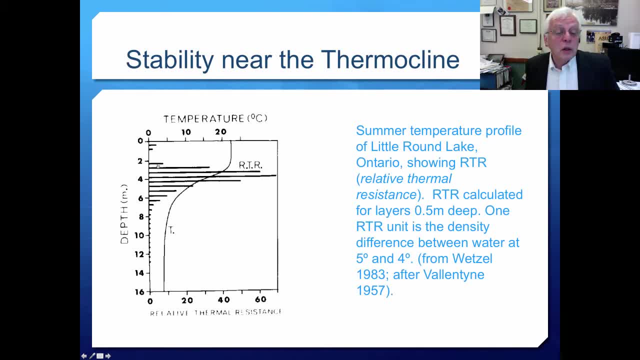 up here. it doesn't take very much. it's not very resistant to mixing- the water column isn't- but when you get down to the thermocline it acts like a fairly strong barrier and in diving in lakes i've actually um, i've actually been able to see um the thermocline by particulate matter. 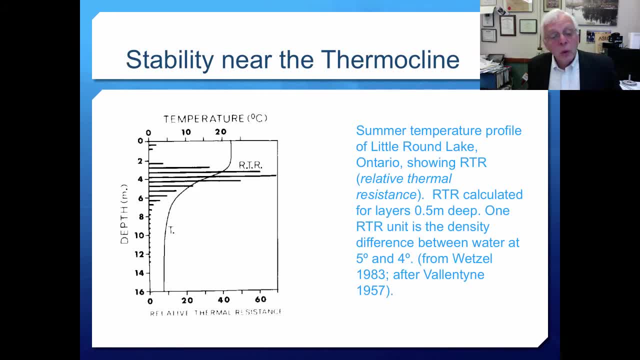 that sits on it, a particulate matter that falls down and won't drop any farther because it is at the same specific gravity as the thermocline. you can observe these things pretty well now. there are different ways of discerning the position of the thermocline, and one of them: 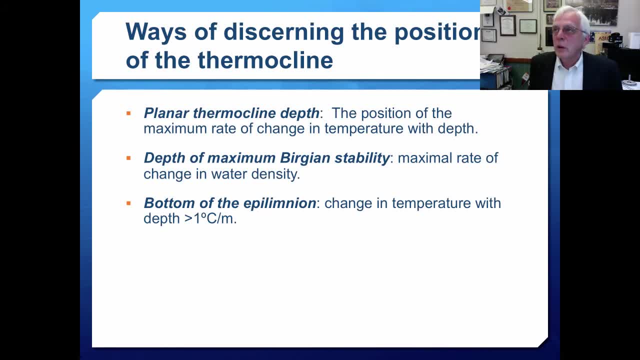 i've just shown you, and this is the depth of maximum bergian stability, or rtr, relative thickness, thermal resistance to mixing, and um, that's the middle one in this, um, in these bullet points, um, and that's, that's a very good way of determining the position of the thermocline. other uh, easier. 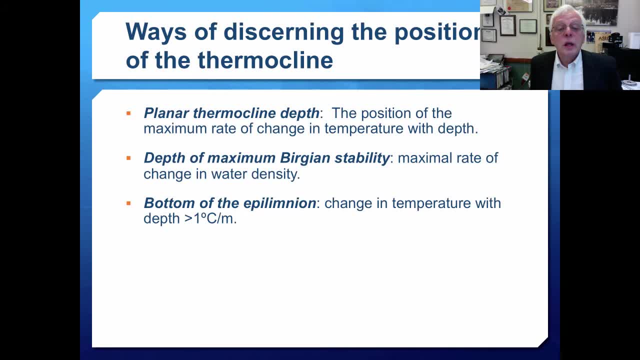 ways would be to look for the planar thermocline depth. this is a position of the maximum rate of change in temperature with depth. now, this doesn't always imply a great deal of of stability. another way to find it and the way we do this often in the field, when we're trying to um determine where 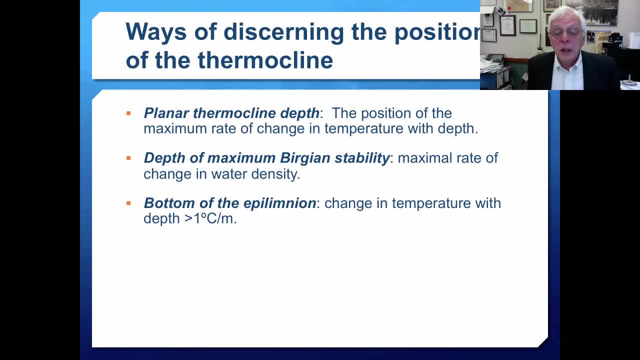 the upper mix zone is is to look for the bottom of the epilimnion. this is uh, the where the change in temperature with depth is greater than about one degree celsius per meter. so there are different ways of doing it. probably the best way is looking at the depth of actual maximum stability. that 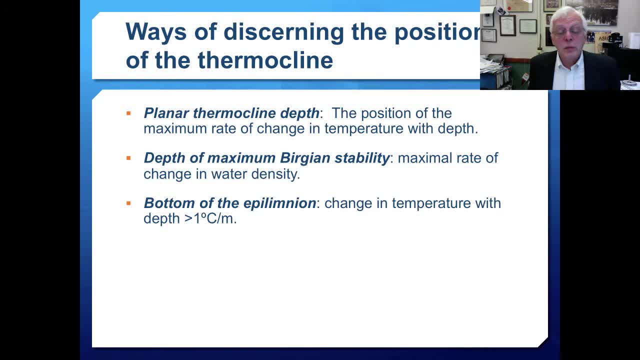 would be the best thermocline, unless of course the maximum stability is not high enough to prevent mixing. but another way to do it easily in the field is look for the um. look for a place where the change in temperature with depth becomes greater than about a degree. 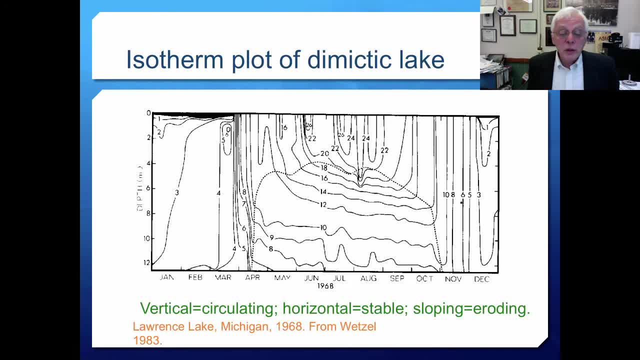 celsius per meter. now here's an isotherm plot- and this is quite important for you to learn how to read, and this is a three-dimensional plot. essentially, what you see on the y-axis again is depth in meters, from zero at the top to 12 meters roughly at the bottom. 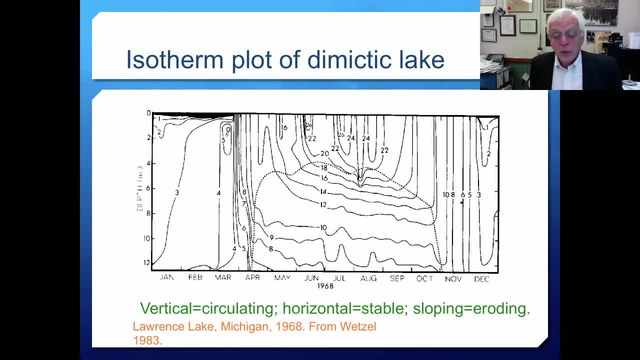 and you see dates. of course this is prehistoric, from 1968, but this is a full year of the years. uh. thermal data from um lawrence lake in michigan, a fairly famous lake. it's been studied quite a lot. now the dashed line is the position in depth of the thermocline and that's calculated. 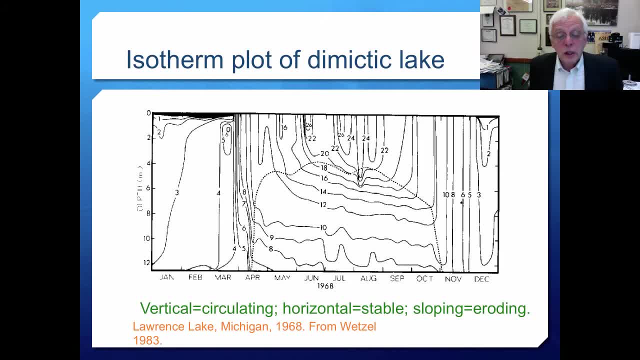 of course, and can be calculated in any of the ways we suggested in the previous slide. okay, now here's a trick in understanding these. these are contours of equal, equal temperature and, for example, you can, you can see, for example, you can see that here this particular isotherm is a 12 degree isotherm, and what this? 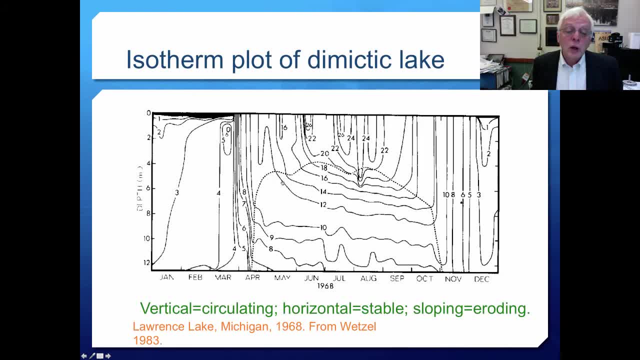 line. descending means is the 12 degree. isotherm is descending into the water column and getting deeper and deeper and that happens as you move through the season. and as you move through the season then the water column warms. you see some fairly big numbers up here. 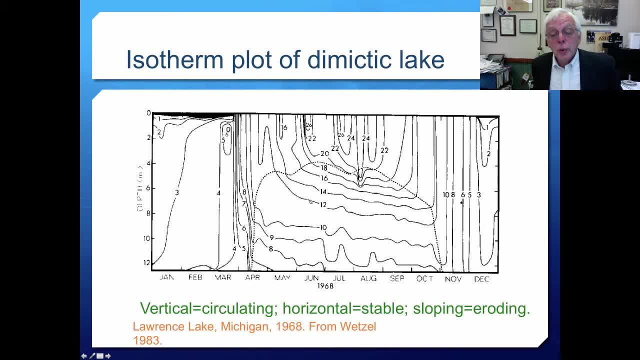 and you get some mixing due to wind and you push down that 12 degree isotherm. a trick to learn in understanding how to read these graphs is that when the lines are straight up and down or relatively straight up and down, that means the water column is mixing fairly thoroughly. 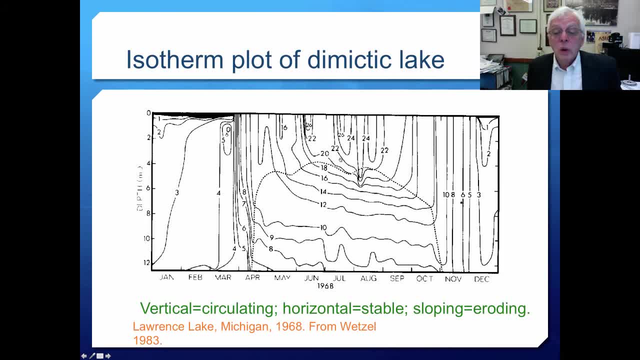 when the lines are horizontal, that means that the water column is stable and this is a fairly uh well water column is stable and stratified. so vertical lines would mean mixing, horizontal lines would mean a stratification, and then you can see it toward the end of the season the lines go from horizontal to vertical and that means the lake is. 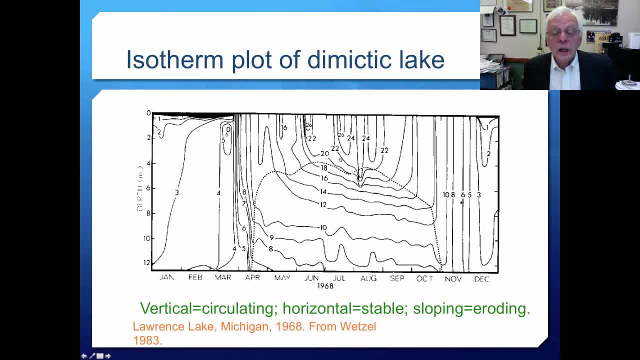 mixing again. now what this tells you, if you've been thinking about it carefully, is: in this particular Lake, there are two periods of mixing. there's a period of mixing in the spring and a period of mixing in the fall. easily discernible here, vertical lines and vertical lines. in the summertime, this Lake tends to be very stratified. now this has. 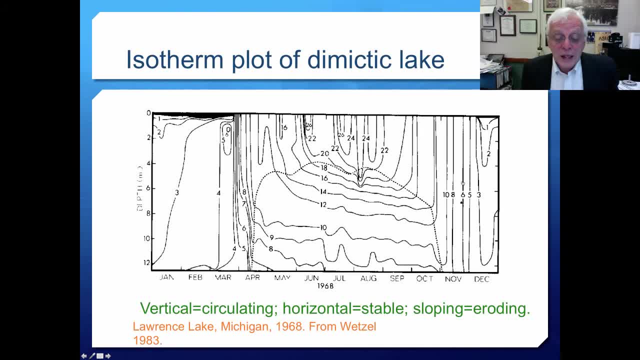 two periods of mixing, so it is what is called a dimictic Lake. it mixes twice per year. you may have heard people talk about overturn of lakes. um, that's really not right, because the water doesn't turn over like the bottom go to the top and the top to the bottom. what happens is it circulates. 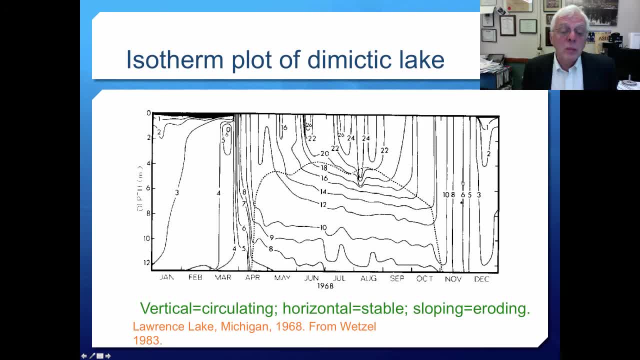 from top to bottom. so in Limnology we prefer to talk about vertical lines, vertical lines, vertical lines, circulation, periods of circulation or mixing of the water column. this is a diamictic lake, has two periods of mixing and then fairly strong stratification in the summer, with a thermocline at about four degrees Celsius a little bit later. 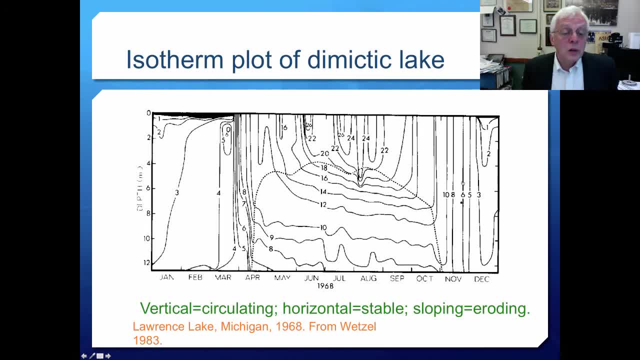 on in the course you're going to learn that. sorry, thermoclines not at four degrees Celsius, excuse me, the thermoclines at about four meters. four meters of depth, okay, so you can see that by running over to this axis and seeing this number four over there. so four meters depth, about 12 feet. 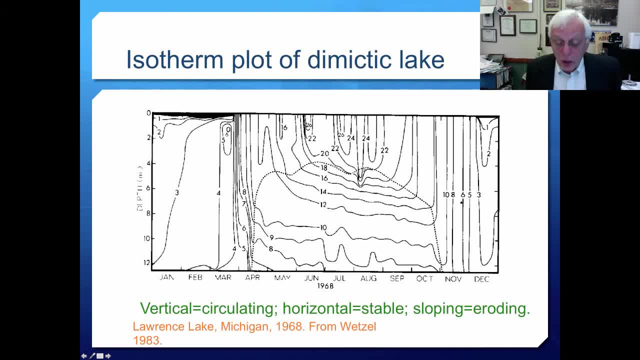 something like that is where you have, where you have, a thermocline. now, what that means, of course, is- and we'll learn this later- when we talk about the physics of lakes- it means we can guess that this is a fairly small lake, or a lake that's oriented crosswise to the wind, or some other factor that would. 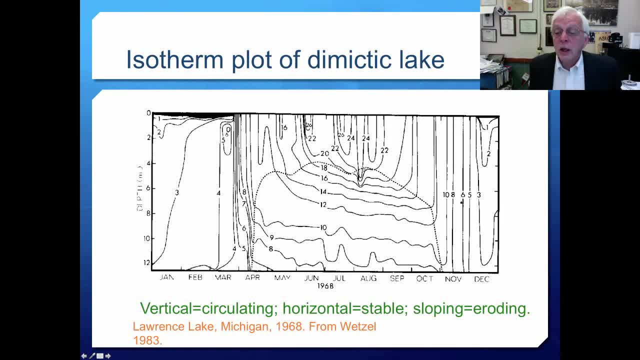 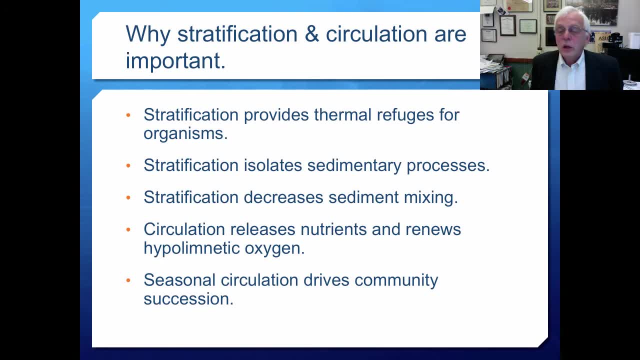 make it mix down deeper, but that we can reserve for another time. now a a. here are some reasons that stratification and circulation are really important. stratification provides thermal refuges for organisms because it keeps the water cool down at the bottom rather than letting it hit those. 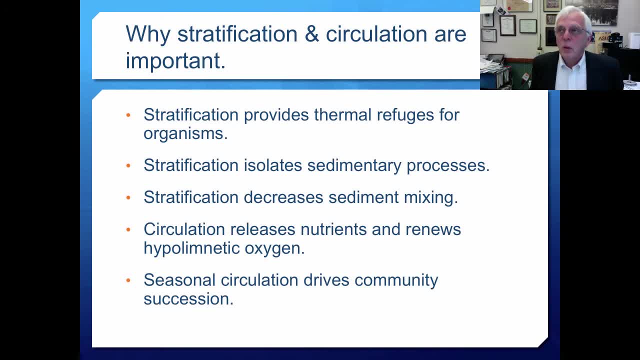 relatively high extremes, that is to say freezing or let's say 30 degrees at the surface, so it can keep a cool water refuge. stratification also isolates sedimentary processes- pretty important because sediments tend to exude nutrients and other materials and that means in the summer you can keep clear water because you're not. 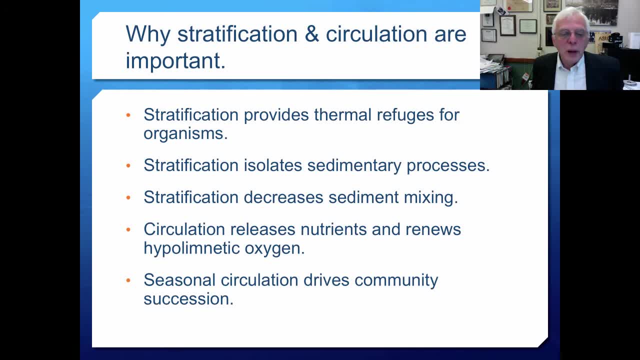 feeding that sediment nutrient material back into the water column. also, stratification decreases sediment mixing and sometimes you'll get enough wind energy mixed into a lake that it will actually kick up the sediment on the bottom, and so stratification keeps that sediment mixing fairly low during periods of stratification. another important aspect is sort of the the 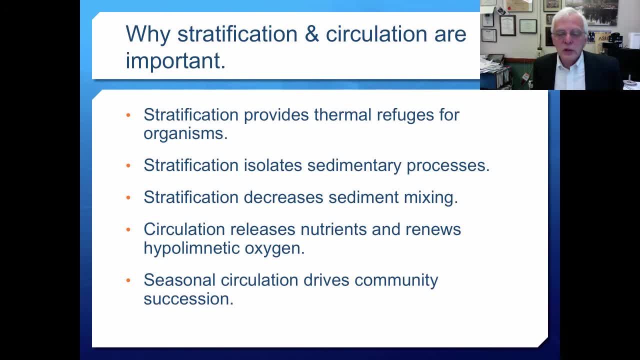 inverse of this circulation is very important because it releases nutrients and renews hypolimnetic oxygen. you can imagine that once you've established a thermocline, the oxygen concentration- that's in the amount of oxygen that's in the hypolimnion- is pretty much fixed. no more oxygen is coming back in, and so it. 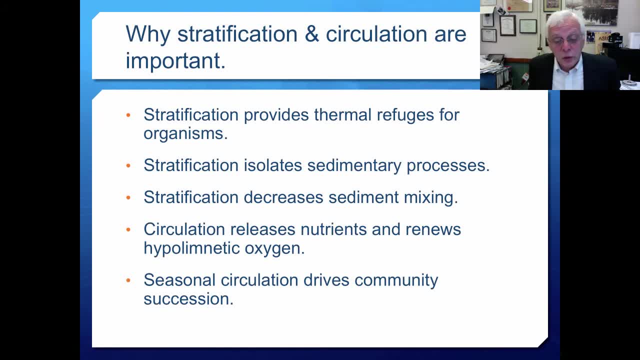 can be depleted by decomposition, by other, by various respiring organisms, and at that point, if you kept it always isolated from the atmosphere, unless you have some primary production down there, you're not going to renew the oxygen and things will tend to die. so circulation releases nutrients and 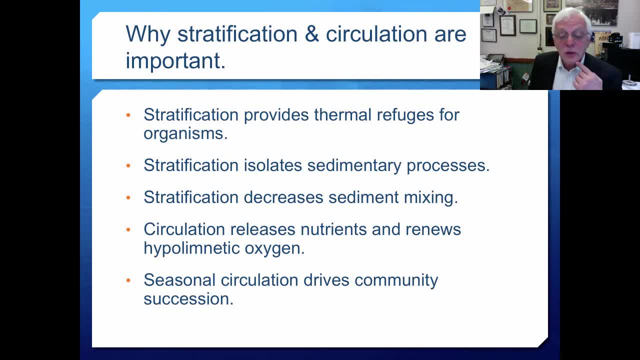 renews hypolimnetic oxygen. also, seasonal circulation drives community succession. you may have noticed in looking at lakes it sometimes you get big blooms of algae, sometimes you don't. sometimes the water has sort of brown kinds of algae in it and so on. it's this, a seasonal circulation pattern, that makes the 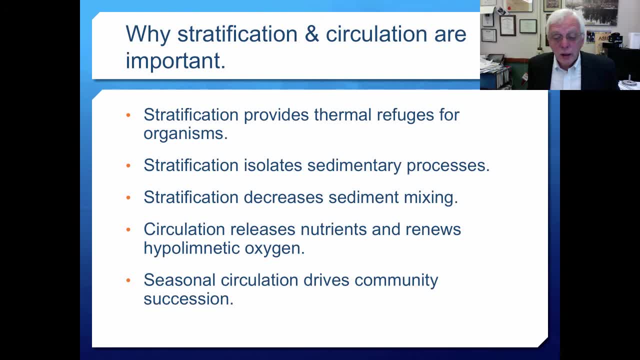 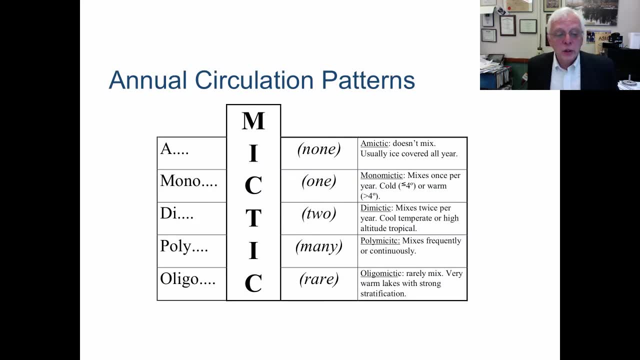 community. change over the season, uh, and it's driven by nutrients and uh, and, of course, by light and temperature. now there are different kinds of circulation patterns and i already talked to you about dimictic lakes. uh, dimictic meaning mixing twice. you can also put the 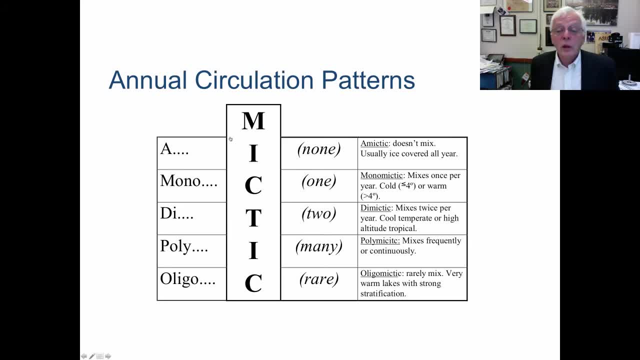 a on the front of it, as here, and make the word amictic. amictic lakes do not mix, and these are lakes that are usually ice covered all year. uh, you'll see, uh, in some futures slides, that there are some kinds of lakes that are not ice covered. 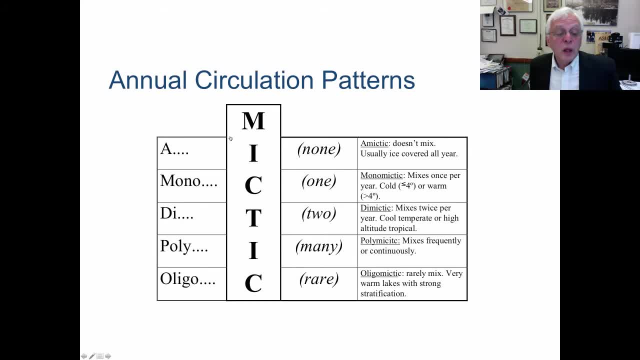 that are amictic, but that has to do with chemical stratification. now, monomictic lakes are those that mix once per year and we have two kinds of uh monomictic lakes and these are cold monomictic or warm monomictic lakes. 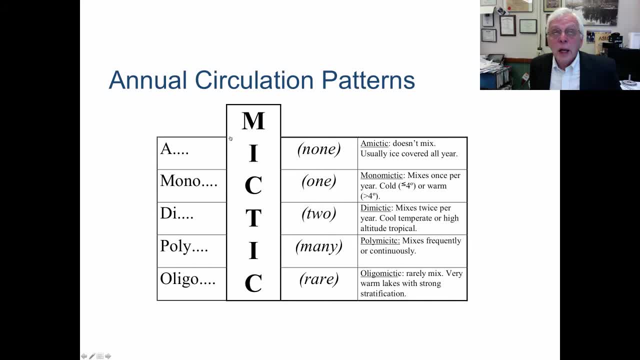 now. cold monomictic lakes usually are those that uh will lose their ice cover briefly. warm up slightly so the entire water column becomes four degrees, mix top to bottom and then regain ice cover. warm monomictic lakes are usually those uh lakes in areas where there is a 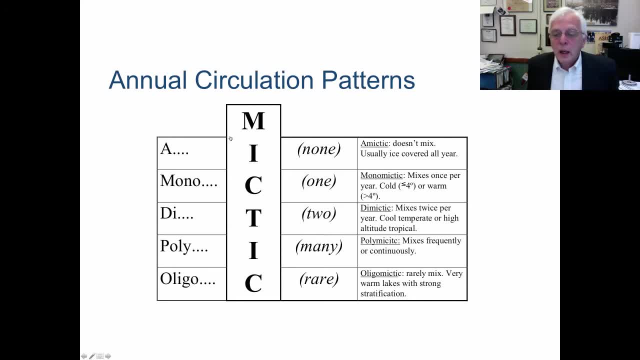 typhoon season or a stormy period, that uh will change the water temperature uh and the amount of water coming in and the amount of wind, and these are lakes that are usually stratified. you remember that in warm systems, because of the specific, miraculous uh characteristics of water, 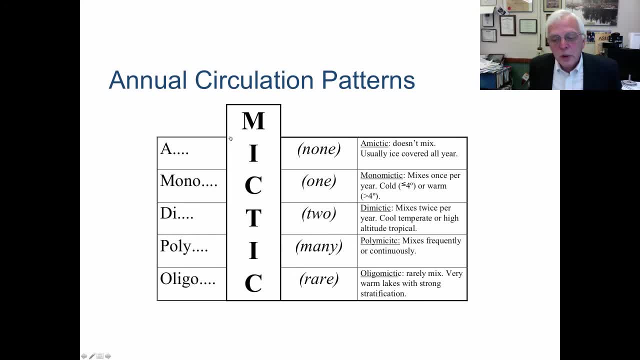 uh, we can have strong stratification, even though temperature differences top to bottom may be small, and then we'll have an input and a cooling- input of water and cooling and wind mixing. and sometimes these lakes in the tropics will also be monomyctic. so we have cold monomyctic and warm monomyctic lakes, diametric. 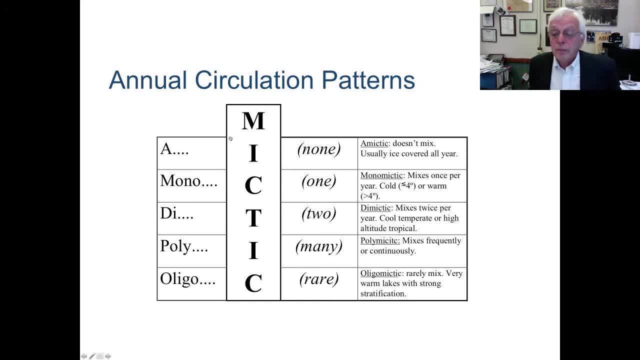 lakes are those that mix twice per year, and these are are usually found in cool temperate zones or high-altitude tropical systems that will actually mix twice a year and stay stable the rest of the year. polymictic lakes are those that mix a lot- poly meaning many and- and these mix very frequently or even 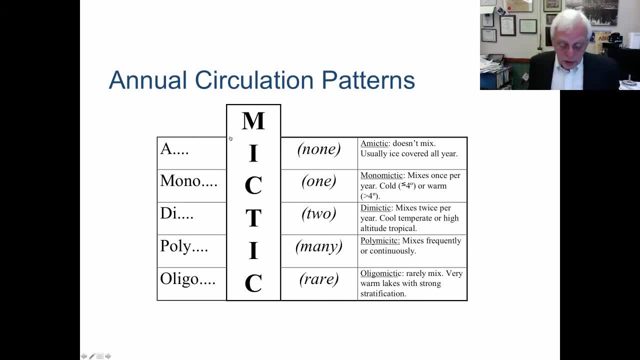 continuously and we're seeing a lot in the, even in temperate zones, seeing a lot more polymictic lakes, and we used to. simply because the climate is getting warmer and actually seasons are becoming stormier, the final kind of circulation pattern we see in lakes would be oligomyctic lakes and oligomyctic lakes rarely mix. they're. 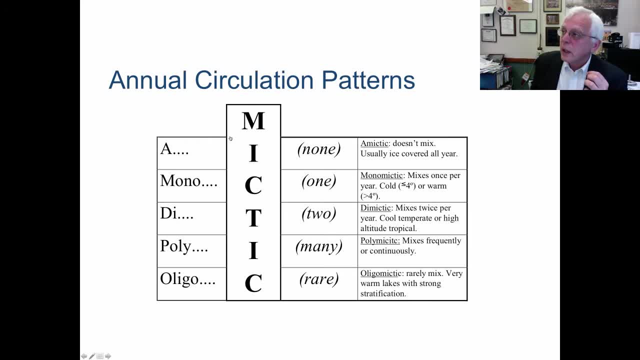 usually very warm lakes with strong stratification and only rare stormy periods, or in some cases they may be chemically stratified lakes that only mix when there's a massive amount of energy input. those are the various kinds of mixing regimes that I'd really like you. 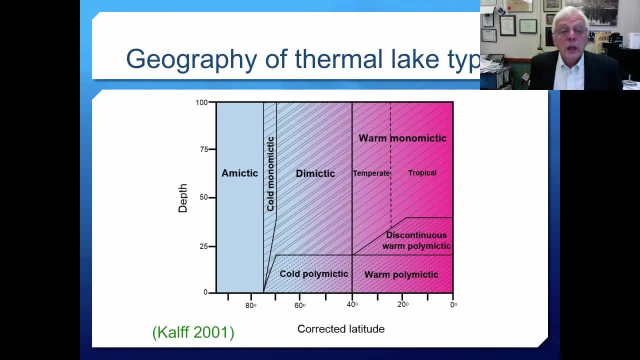 to learn and understand now if you look at the geography of thermal lake types. so we've already talked about this, really, but there is an effect of depth, of course, and altitude of latitude, sorry, and deeper lakes, of course, tend to mix less because you're dealing with a much longer, taller water column that you have. 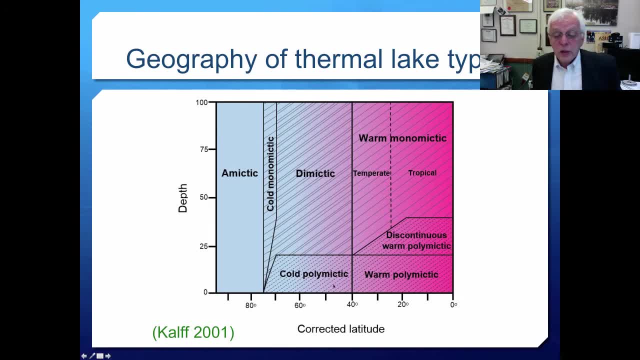 to mix top to bottom and as we move through various latitudes. here's 40 degrees latitude. actually, as I'm recording this, I'm in the state of Iowa, which is just a little bit north of this of that 40 degree mark. that's sort of. 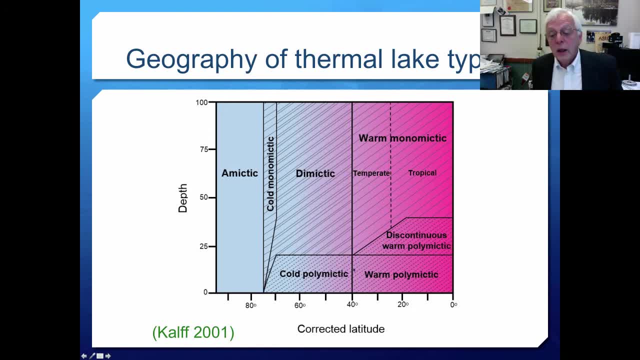 the area sort of on the boundary between sort of where we get warm polymictic lakes and cold polymictic lakes, and that has to do with temperature and the strength of stratification. in warm areas or in sort of low latitude zones, the when the lakes get deeper and deeper. 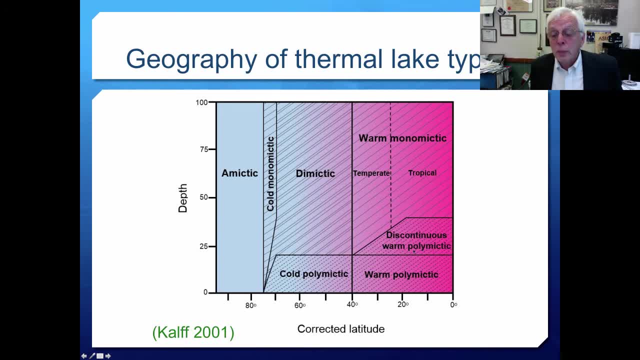 they tend to get to be discontinuous- warm polymictic lakes, because it takes more energy to pour in there in order to mix the system. or we may move into warm monomictic lakes, which again are those that will mix when there's a big storm. 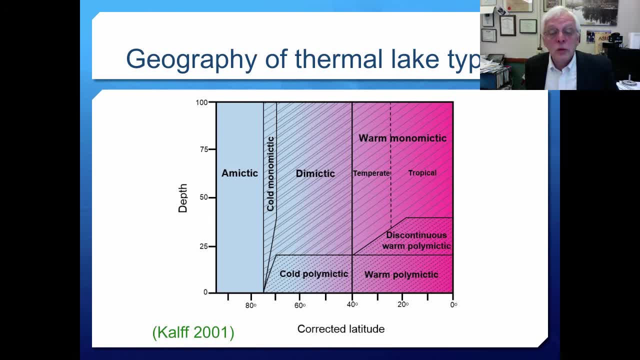 or a cooling period often associated with monsoons. over at the left-hand side. here we see the higher latitudes. these are cold, polymictic if very shallow, but mostly diamictic if they have substantial depth. and once we are moving into the very high latitudes, up at 70- 75 degrees north, then we will see. 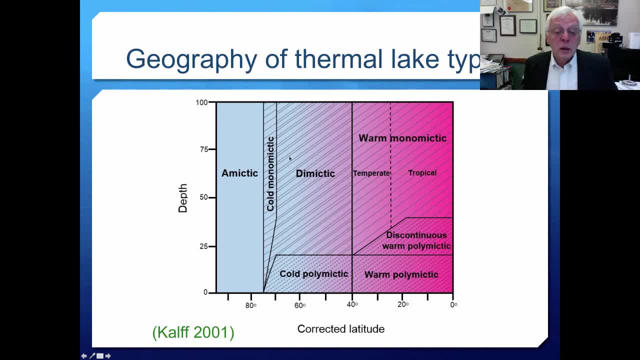 some cold, monomictic lakes, and this depends on the lakes becoming ice-free for some period of the season, and then when we get farther north, lakes are usually very, are usually ice covered and so will be amictic. This is a figure from the Calfe book. actually, this is redone for the new book. 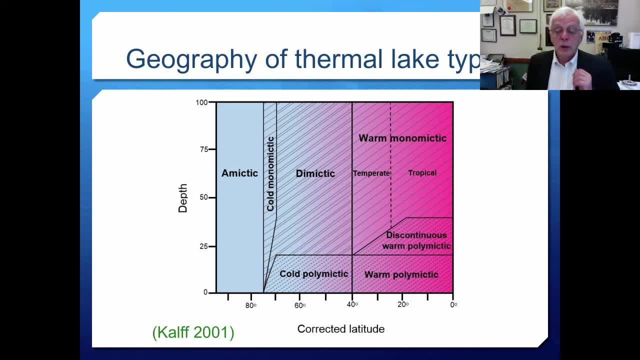 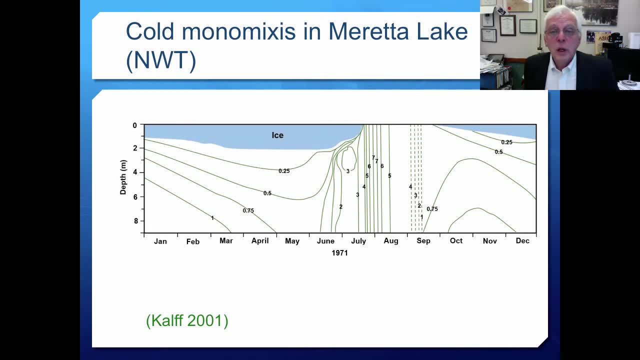 that will be coming out, I hope, if it has not already done so. Now here's. here's an isotherm plot for a cold monomictic lake. this is Maretta lake in northwest territories of Canada, and here you can see at the top. 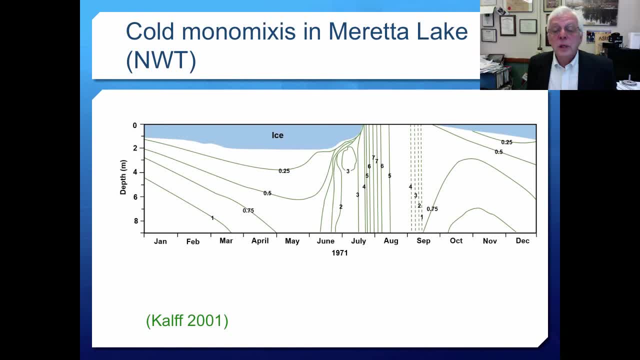 the ice cover is substantial. ice covers a meter and a half of ice and it's. the system is quite cold, except when ice cover is lost and then the temperature moves up to it mixes after ice cover is lost and and the lake mixes top to bottom and then begins. 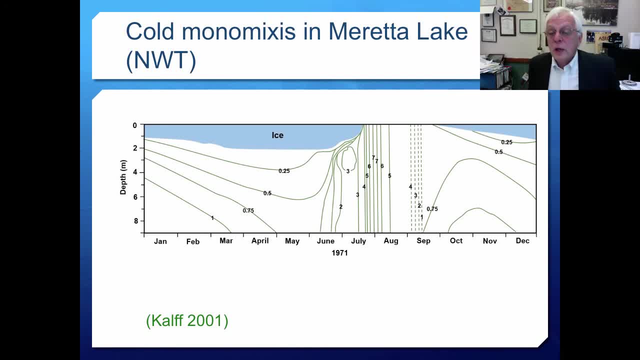 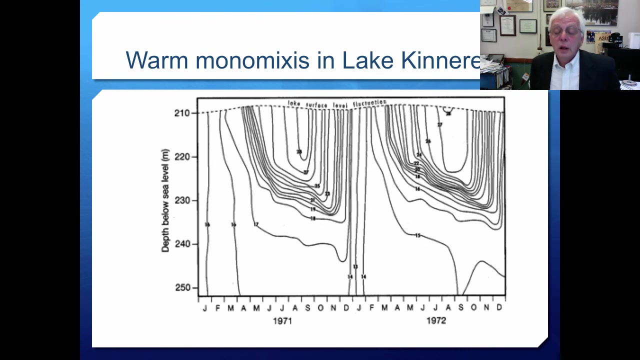 to have very intermittent mixing and then regains ice cover again, in which case it's stratified for the winter again. you can tell periods of stratification by the relative degree of horizontal lines or vertical lines, vertical lines being mixing and relatively horizontal lines mean stable or stratified. here's a warm, monomictic lake in the. this is Lake Kinneret, I think, which 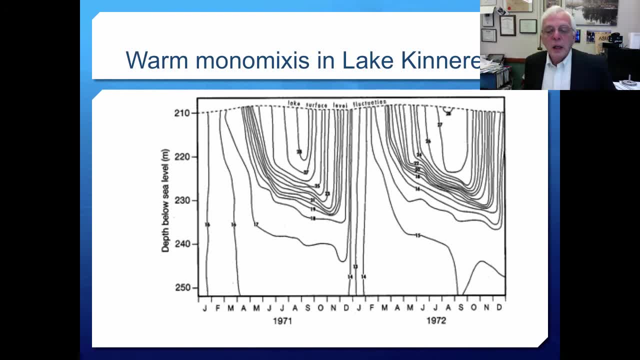 is, I think is called sometimes the Sea of Galilee. and now you. the numbers are quite fuzzy. I'm sorry on this particular plot. I maybe made it a little bit too big, being overzealous, helping, hoping to help you be able to see, but the numbers up in this region are at like 27 and 28 and you know already. 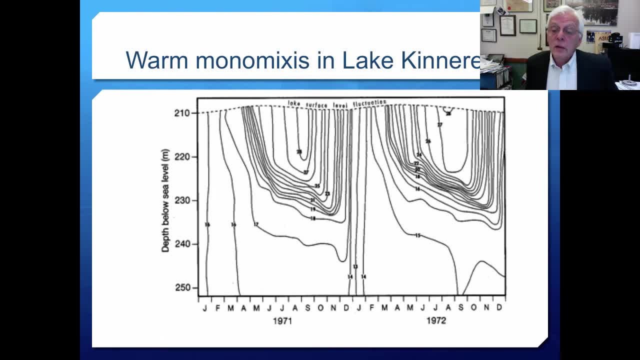 that because of the heat of vaporization of water- high heat of vaporization of water- we're not probably going to go much higher than about 30. so this is about as warm as you get in the world, and what you see here is a stormy season in January or February, in which case the lake will mix top. 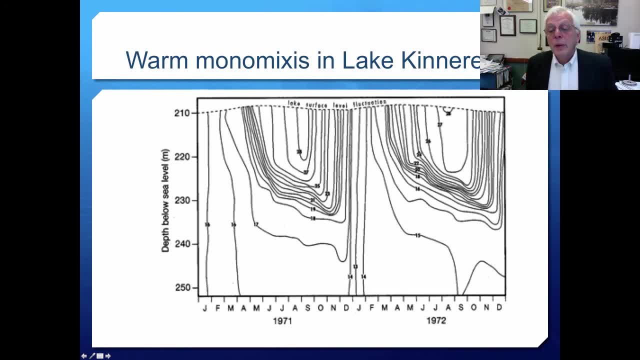 to bottom and gets quite cool. it's replaced by a period of a period of stratification, with the thermocline descending as the season progresses, and this is a little bit confusing. the depth over here this is height depth below sea level. so this entire lake is many meters below sea level in which is very odd, but it's also a very salty sort. 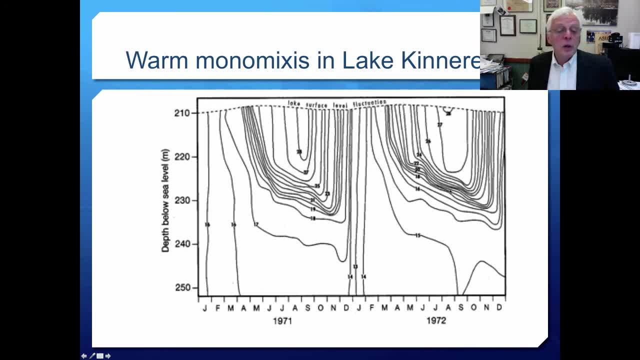 of lake, and so we've, we've got stratification at some depth or somewhere in the neighborhood of 20 meters, descending down to a descend, sending down to about 20 meters, and then, in the stormy season, this is a warm, monomictic lake, and then, in the stormy season, this is a warm, monomictic lake, and 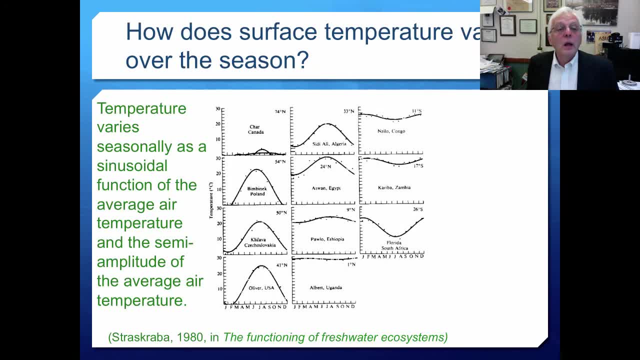 so stratification is lost. so we might think about surface temperature, and surface temperature varies seasonally and it varies seasonally as a sort of a sinusoidal function of the average air temperature and the semi amplitude of the average air temperature. so it's a. basically looks like a. 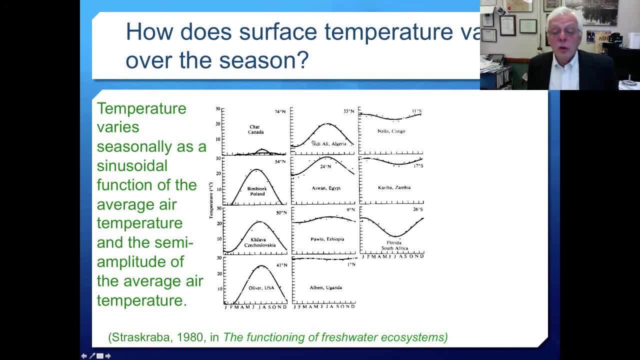 sort of a sine curve, but more or less pronounced depending on where you are in the world. clearly, if it's moving north or west along the equator, it's usually a really nice design. it's a really nice linear between the polar in the north and the south and the east and down around the equator. 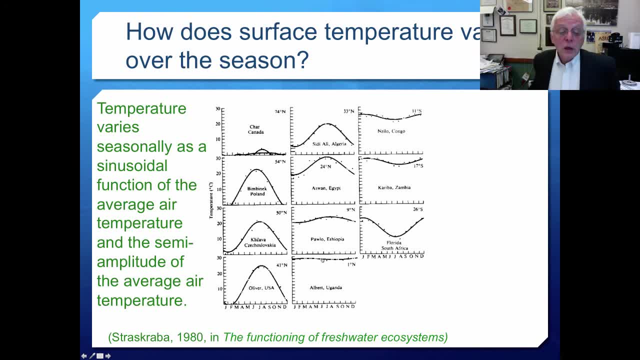 down. this is Lake Albert in Uganda. it's a one degree north of the of the equator. there's not much seasonal variation and temperature at the surface is almost always constant. here we have a lake at 41 degrees north. I think. this is Oliver Lake. I think is in the state of New York, and so 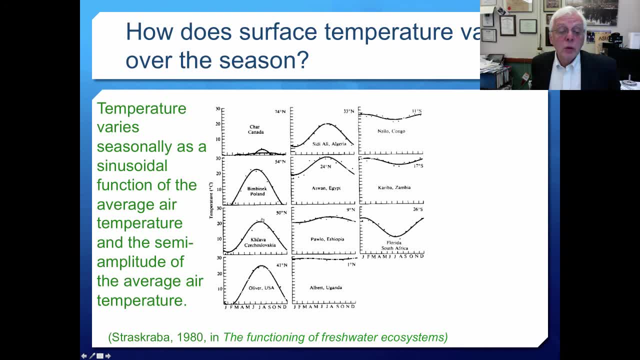 you can see here the temperature gets actually quite high at the surface in the summer and very low, of course, in the wintertime. moving northward down in the north and south, more northerly, we still get some pretty high temperatures in the summertime, but extremely 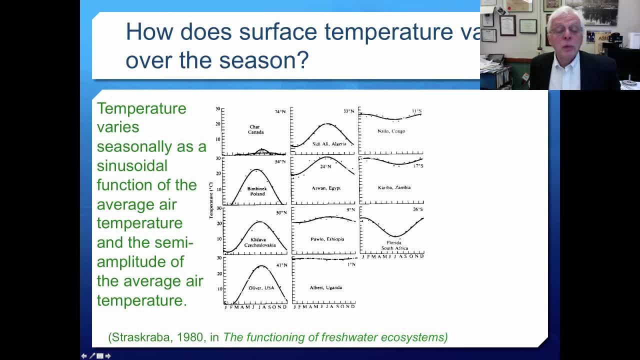 low temperatures in the wintertime, Until you get to something like Char Lake at 74 degrees north, and this would be probably a cold monomictic lake. you get a little blip in temperature, sometimes in the summer, and sometimes it will stay frozen all winter. Likewise, you simply 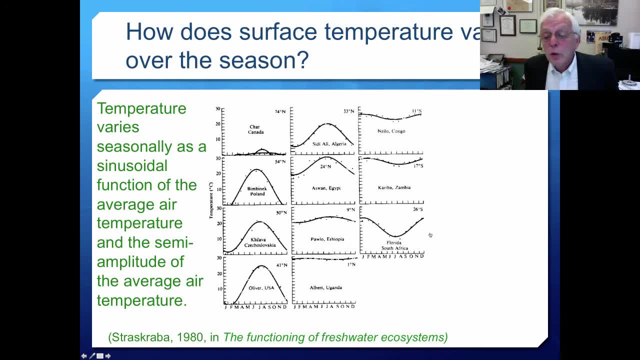 invert everything when you move to the southern latitudes. invert these sinusoidal curves. Bottom line on this is that the temperature can be predicted at the surface pretty well and even in the temperate zones and very high latitudes we'll often attain quite high. 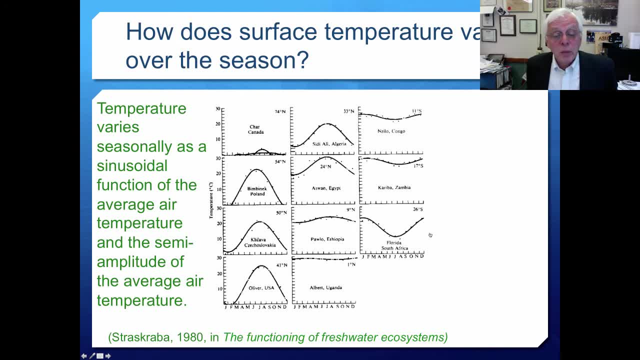 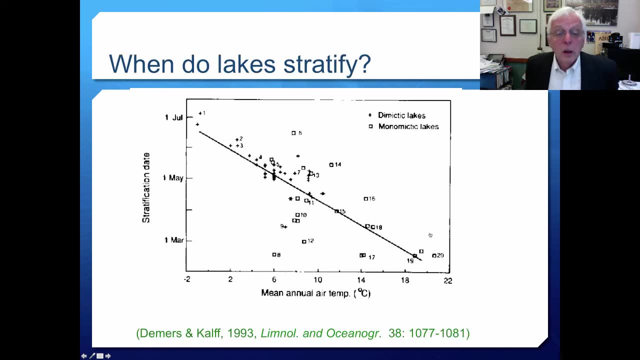 temperatures, and the differences among these periods of stratification would be the temperature and duration of low temperature In the cold period of the year, that is, the wintertime, when ice cover is probably attained. So a question that's often asked is: when might we expect lakes to stratify? 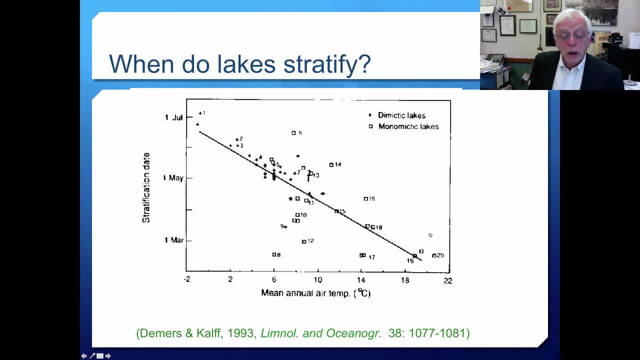 The purpose of showing you this graph? well, purposes are a couple of things. One of them is to show you that it can be kind of fuzzy, kind of a relationship. On the y-axis you see stratification depth When you have the first date and on the x-axis the mean annual air temperature. but you also 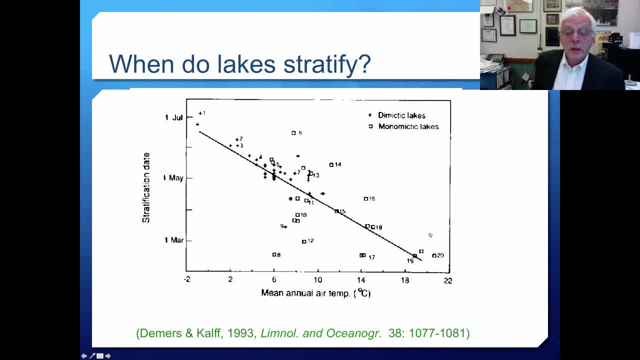 see quite a difference between diamictic lakes and monomictic lakes Now, as you move, these are pluses up here. those are diamictic lakes and you'll have a lot of diamictic lakes until you get to a mean annual air temperature of about 8 degrees. 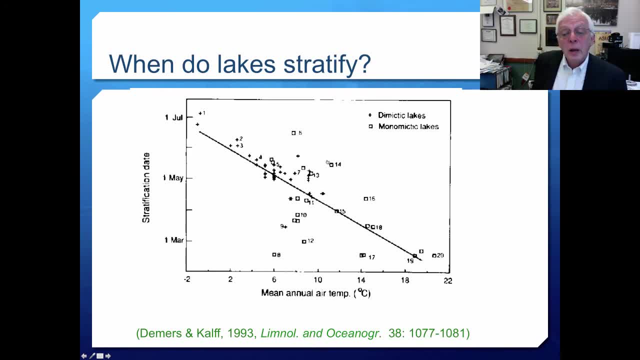 Celsius. Then you begin to have monomictic lakes of the sort of warm monomictic variety, and the stratification downtime date may in fact get rather fuzzy. Bottom line on this is that as long as we're in a diametric system in the temperate zone, 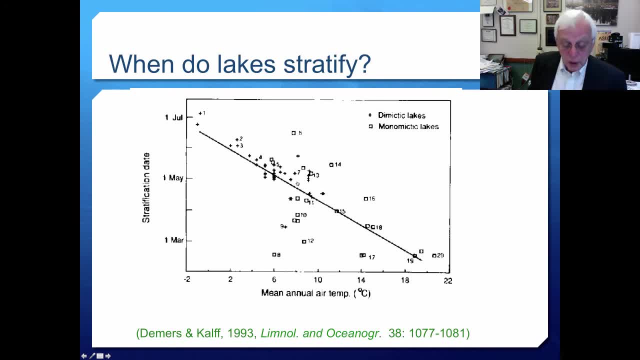 we can predict the stratification date, But it's driven by temperature, So you can think what would you expect based on climate change. Would these things be changing? And the answer is: for a given latitude, of course. as temperature warms, they will tend. 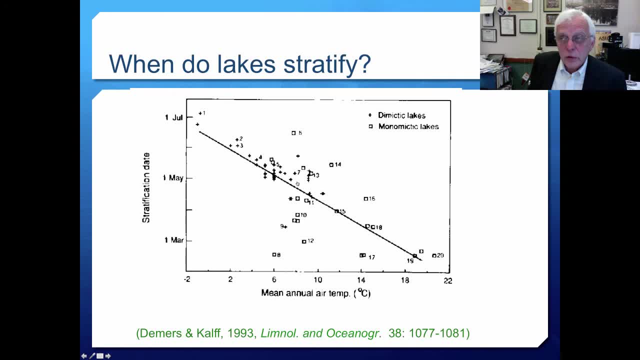 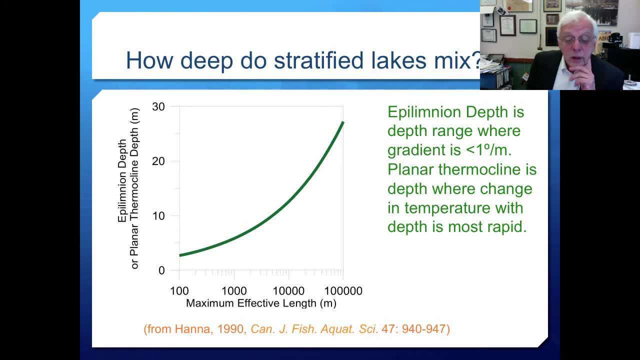 to have an earlier and earlier date at which ice cover is lost and stratification is attained for the summer period. Now, I mentioned a little while ago the depth of stratification. We were looking at Lawrence Lake and said, OK, that well stratifies in the summer at about four meters. 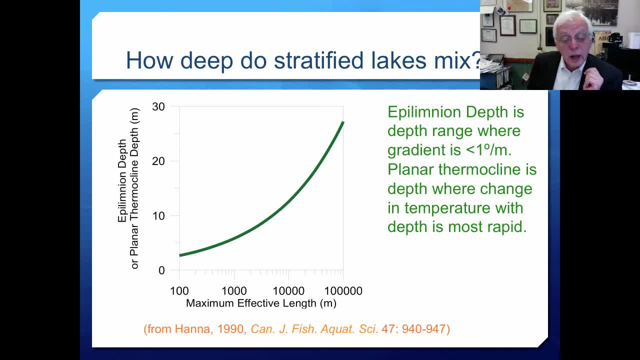 And so I said: well, it's a pretty small lake. This graph shows on the x-axis- This is from work by Micheline Hanna back in the 1990s, where she shows a maximum effective length in meters 1,000, being a kilometer. 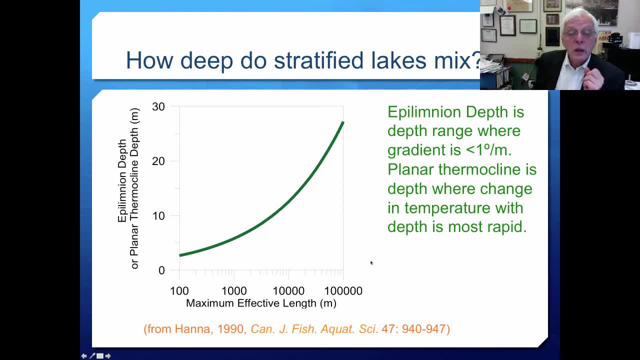 And this being 10 kilometers and 100 kilometers over here, so very big lakes. Essentially the epilimnetic depth, or planar thermocline depth, tend to increase as the lake gets bigger And these are in meters. So I said a little bit earlier that in lakes of a moderate size, 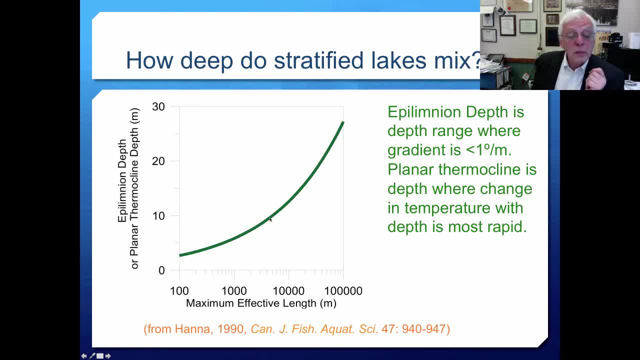 you can expect to find a thermocline at around 30 feet or 10 meters, And that would be for a lake of a kilometer to 10 kilometers in size, Clearly in large lakes and lakes like Lake Superior, for example, which are very deep well, 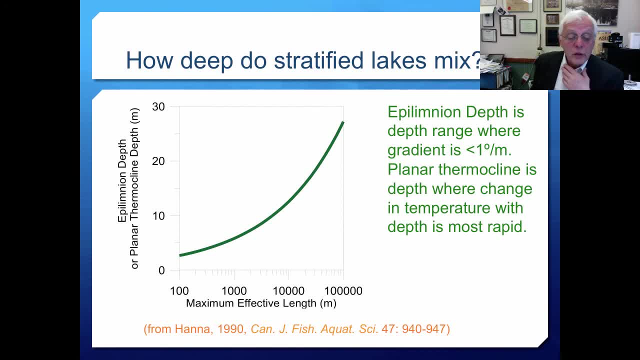 and Lake Baikal in Russia being extremely large, they will have very deep thermoclines. Epilimnetic depth tends to increase as lakes get bigger And little lakes stratify at a shallower depth. There are lots of models for predicting. 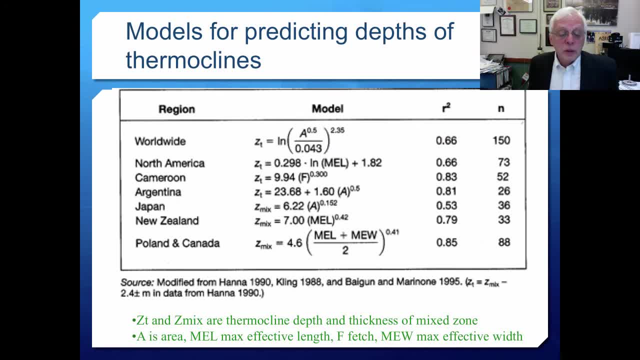 depths of thermoclines, And these are just reviewed here. But what I'd like you to see from this are the variables that tend to drive the depth of thermocline mixing. These would be the Z here. Z for limnologists is almost always or Z. 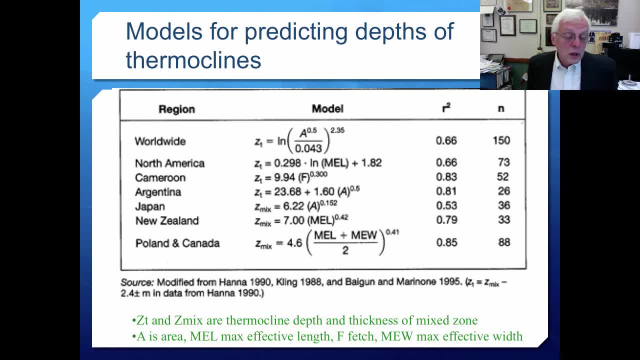 as I would normally call it in Canada. Z is depth, almost always, And Z sub T and Z sub mixing are the thermocline depth and the thickness of the mixed zone. So those are the variables we're trying to predict. A on the right sides of those equations. 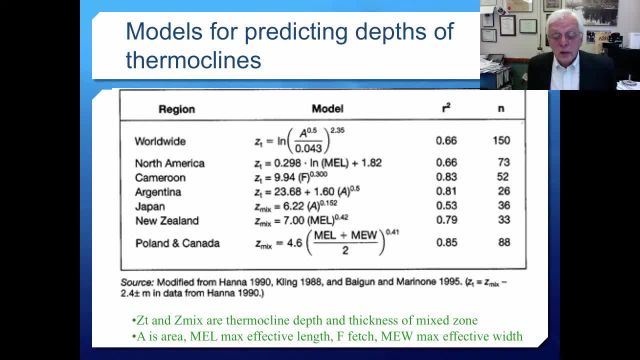 is the area of a lake. MEL is the maximum effective length, F is fetch, And that's how far the wind can work on the water, And MEW is the maximum effective width. What you can see from this is the depth of the thermocline. 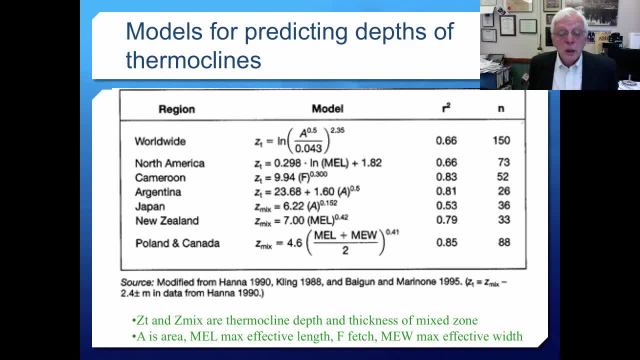 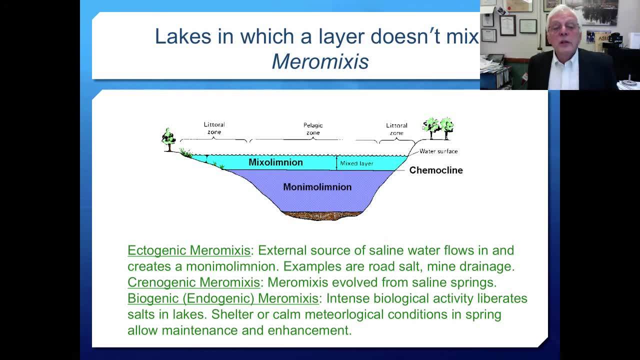 is a fairly clear function, with some predictability of the size of the ecosystem You're discussing Now. the last kind of lake I want to look at here is lakes in which a layer doesn't mix at all, And these are meromictic lakes. 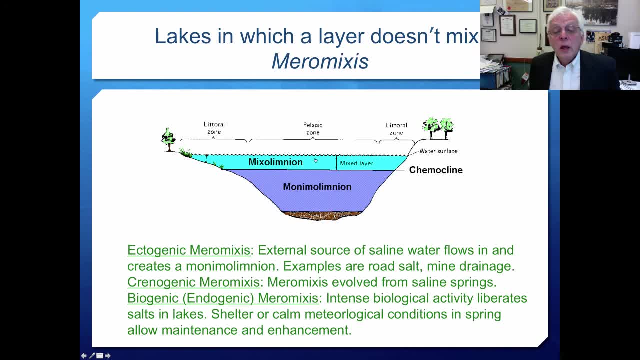 Now meromictic lakes. the layers are called something different. The upper layer is called the mixolimnion And instead of being separated from the bottom water by a thermocline, it is separated by a chemocline. 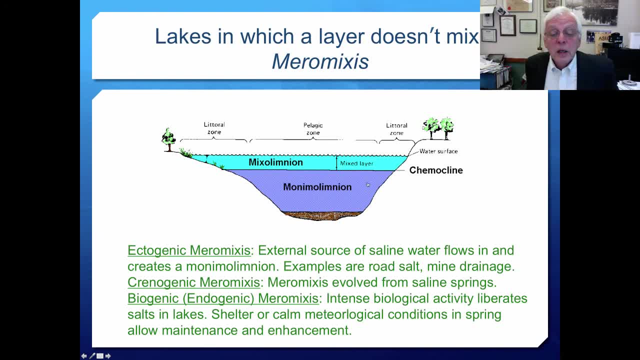 And below in what we would normally call the hypolimnion. That water is called the monomolimnion Now the various kinds of meromictic meromixis, and they are formed by different kinds of processes. 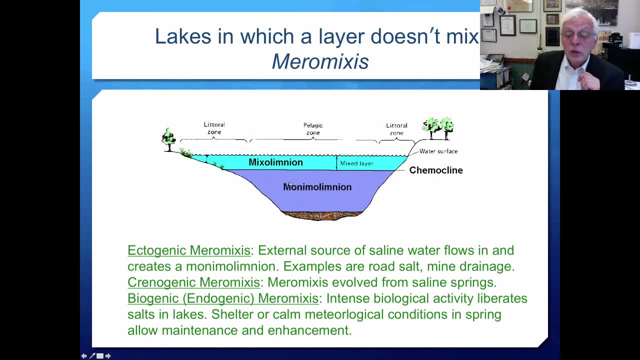 Ectogenic meromixis would be when external sources of saline water flows in and creates that monomolimnion or very stable layer down at the bottom. And we see this often with road salt drainage, with mine drainage and so on where very saline water flows. 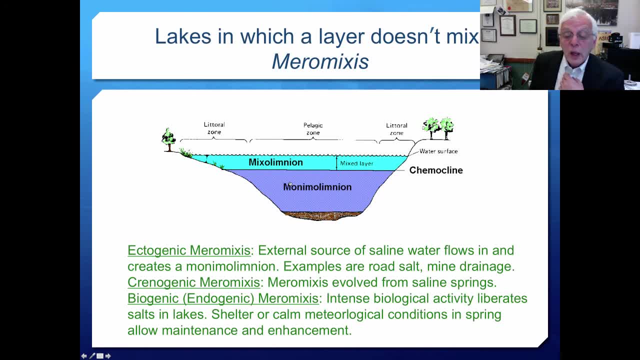 in from the out. Cranogenic meromixis is a meromixis that's evolved from saline springs and their activities, And biogenic or endogenic meromixis is where intense biological activity liberates various kinds of salts in lakes and creates an area that 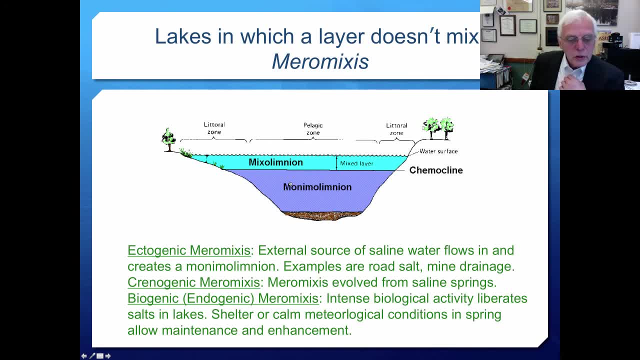 is relatively stable due to the production of salts from the inside. They're endogenic And these usually require something like shelter or calm meteorological conditions in the spring that allow maintenance and enhancement, And I've seen some of these lakes in northern Minnesota, where I work frequently and where lakes are crosswise. 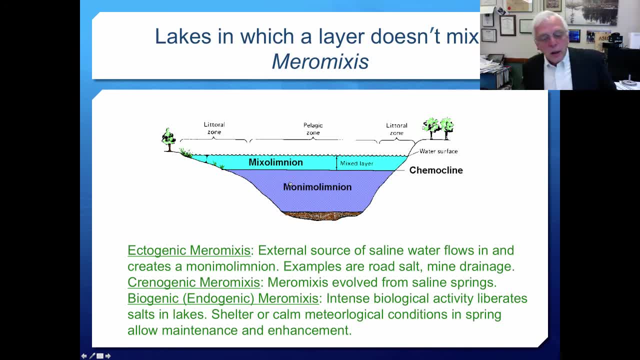 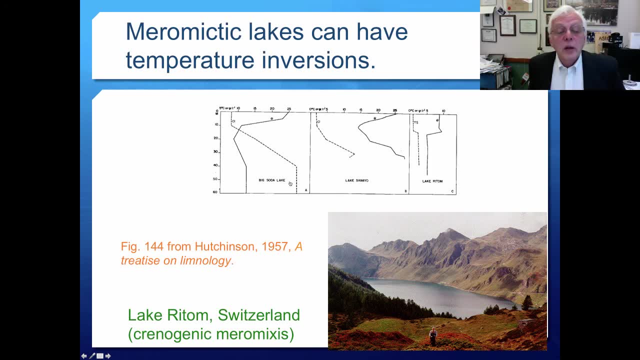 to the winds, very small and quite deep. You'll often find endogenic meromixis. Now, meromictic lakes can have temperature inversions. So the theta that you see in these graphs, or the solid lines, theta is temperature. 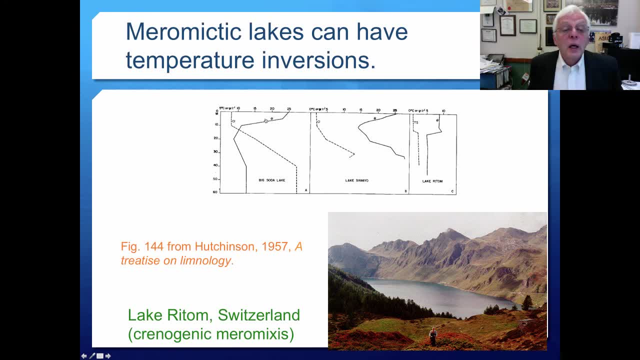 And what you see? in this big soda lake, a lake with some fair depth- we see that the temperature declines in the normal fashion until you get down around the chemocline. Then it begins to warm up in the bottom, And this is because stability is not simply driven by temperature. 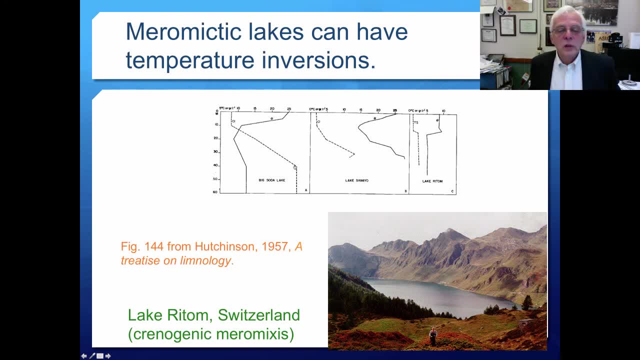 It's driven by salts, And here you see the chloride concentration. You can see it's very salty in the bottom waters and relatively fresh in the surface waters. Likewise, here's Lake Sinmayo. Sinmayo is in Japan And here we have chloride concentration, a chemocline. 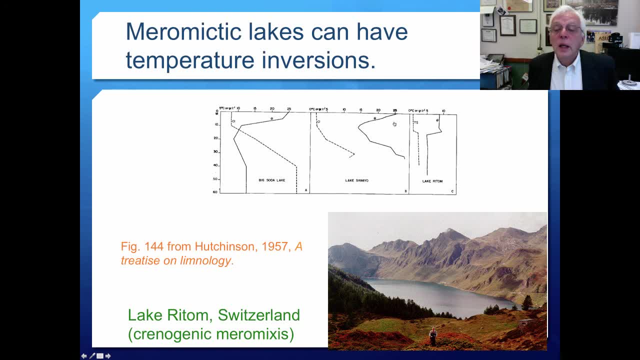 somewhere in this area And we see warming beneath the chemocline, even though the surface waters tend to cool as we decline in the relatively fresh waters at the surface And here we see total solids. This is Rittam, which is shown in the figure below. 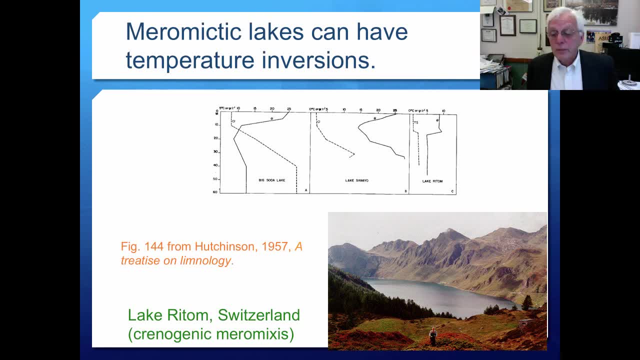 This is an alpine lake, This is chrenogenic meromixis, where there are saline springs And you see total solids, chemocline about here And then here we have very cold temperatures actually at the bottom, but they can show temperature inversions. 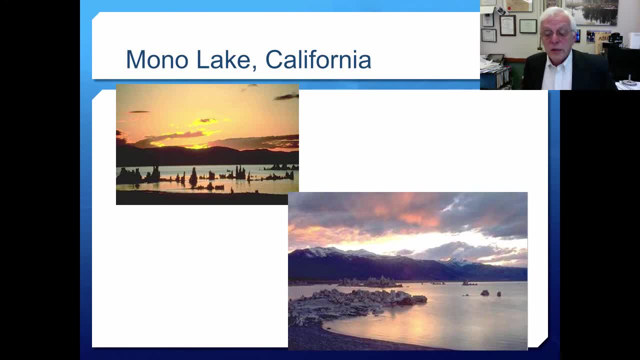 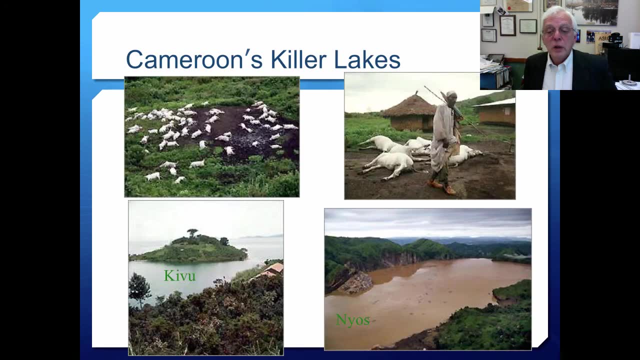 Mono Lake is one of these lakes that shows a lot of salinity and tends to be meromicitic, And sometimes we have meromixis. that generates murderous conditions, And we see this especially in volcanic regions where we'll create a meromicitic layer. 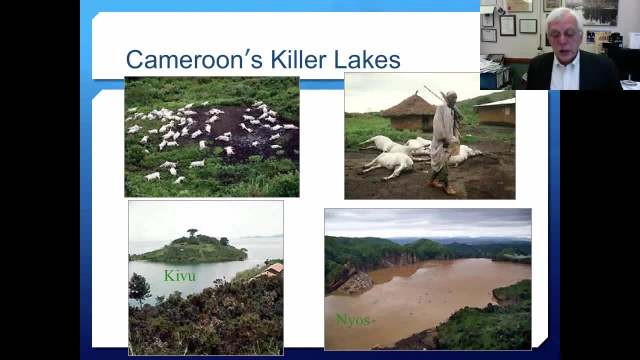 lake, due probably to something like cranogenic maramix. saline springs from volcanic sources, causing salt layers to get very high. Oftentimes there's a very large buildup of carbon dioxide, methane, hydrogen sulfide and other gases down in the monomolemnion, And sometimes due to gas. 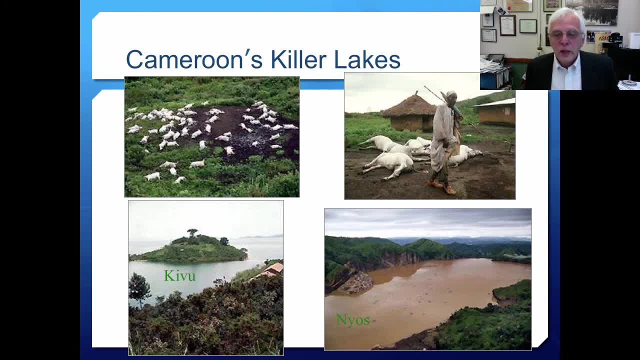 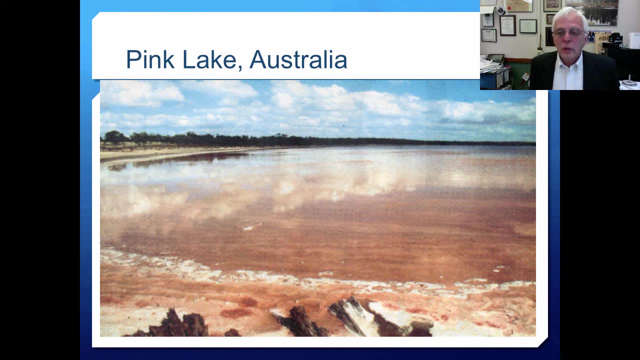 bubbles bubbling up to the surface or other factors, they will invert and mix, releasing all these gases, And they can be actually quite deadly for people and livestock, as is illustrated in these images. Pink Lake Australia is another one of these lakes. You see it's pink because it. 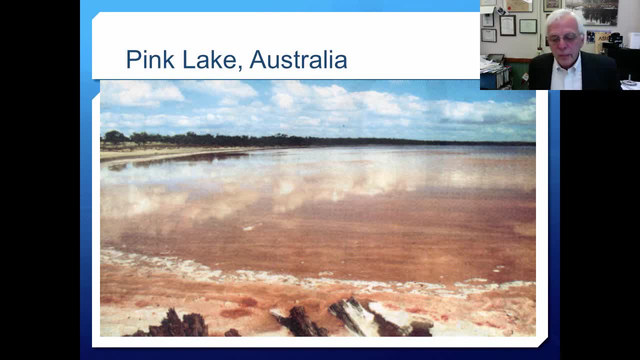 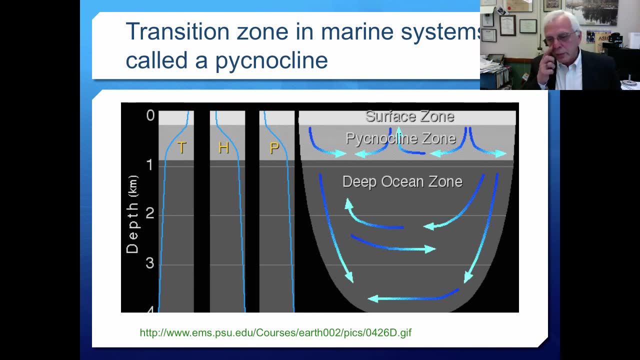 has purple sulfur bacteria in it. This often lives in very saline aquatic systems. Now I'd like to talk extremely briefly about marine systems, Because stratification is slightly different in marine ecosystems. Now we have temperature on. this is a graph in kilometers, not in meters anymore, And this is a graph of temperature and salinity in the deep. 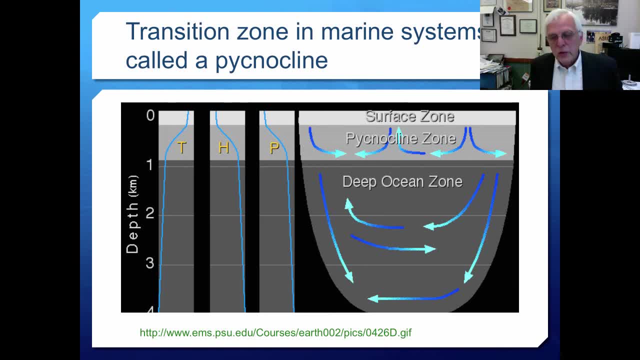 oceans And often because of influx of water at the surface, that fresh water doesn't mix with the rest of the ecosystem. We have a surface zone that's characterized by fairly warm temperatures, but also by relatively low salinities, And the bottom waters are characterized, of course, by very cold temperatures and relatively 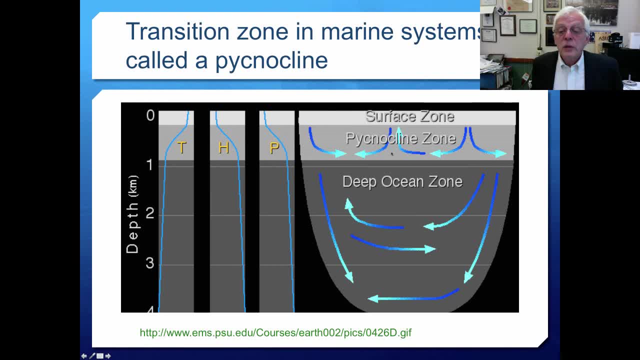 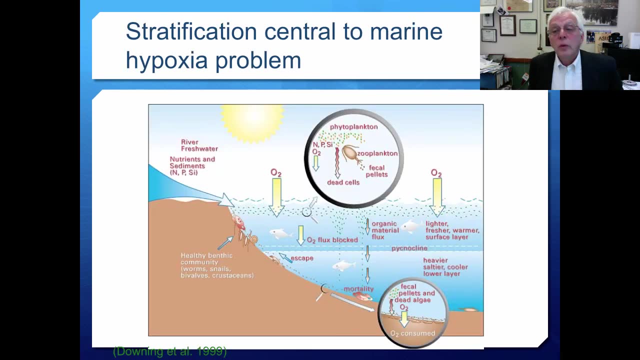 high or ocean-like salinities. These two layers are then separated by the pycnocline zone, which can be really broad, where there's a change in salinity- gradual change in salinity Stratification is central to the marine hypoxia problem, or the dead zone problem that you may have heard about. 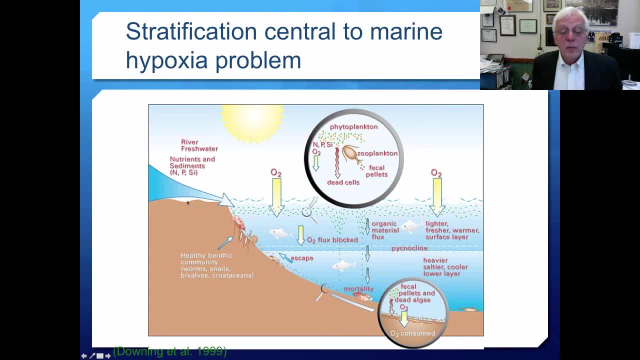